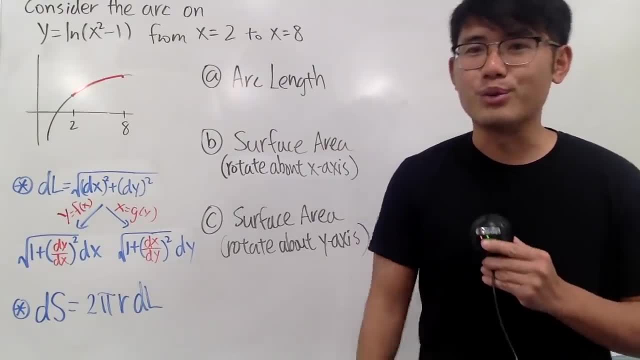 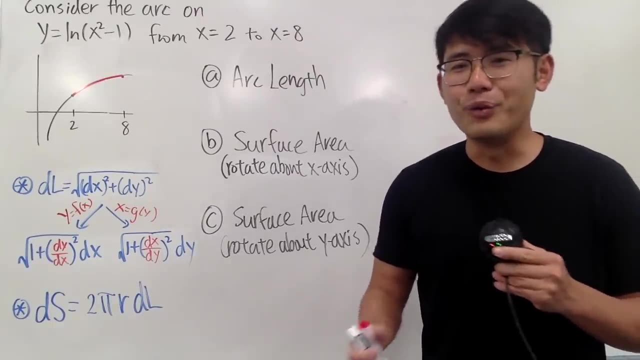 show you guys the setup and you guys can use your graphing calculator to do the integrals. all right. Sometimes when you set an integral for this kind of things, the integrals is either really hard to solve or impossible to solve. So just use a calculator for it and pay really close attention. 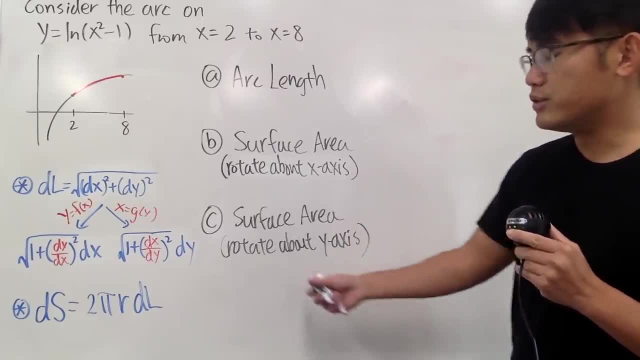 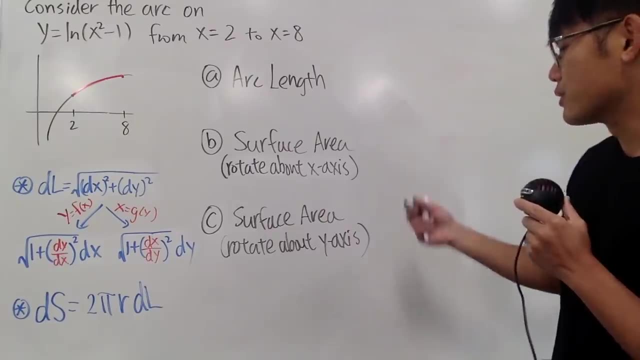 to the details, right, Because maybe on the exam you get just one part for the question and you have to remember the setup for that part And then use a calculator to do the integrals. All right, enough talking, Let's go ahead and do part. 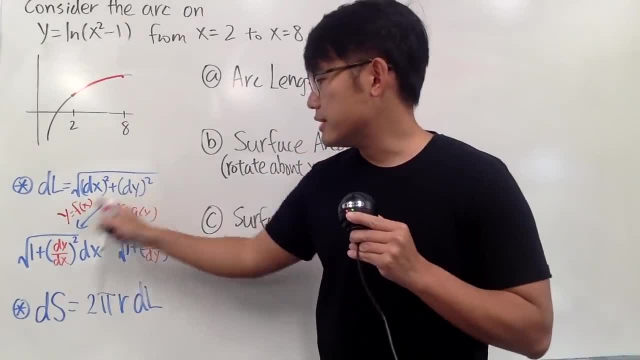 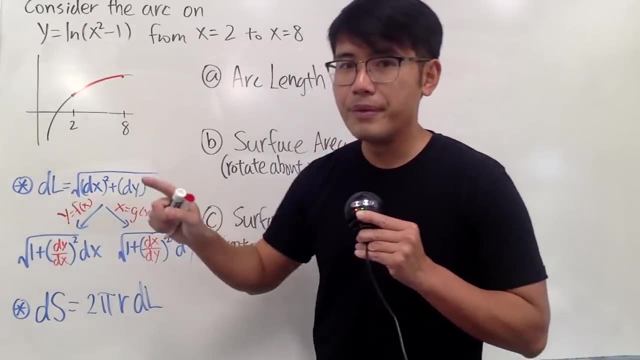 A Well for the r-length formula. as you can see, we have two versions. This right here is just a small change amount in the arc, So I call this to be the dl And it depends on if we have y as a. 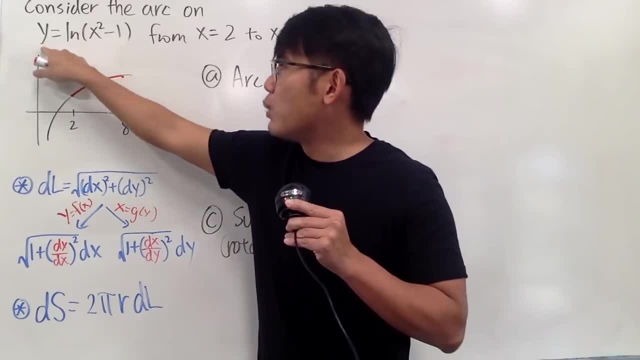 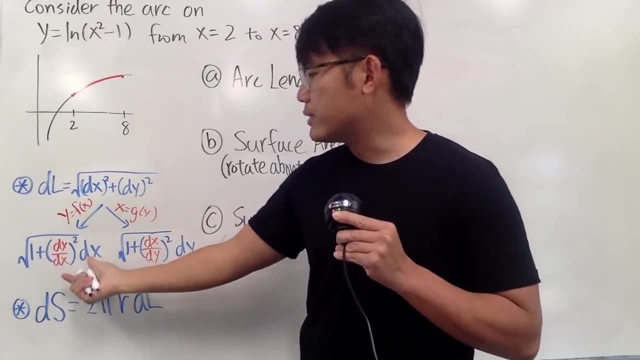 function of x or x as a function of y. In our case we have y as a function of x, so we'll use this version for it. Notice, I just have to factor out the dx squared and then do some algebra. 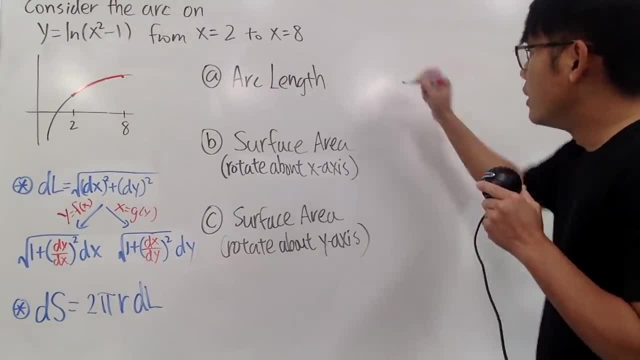 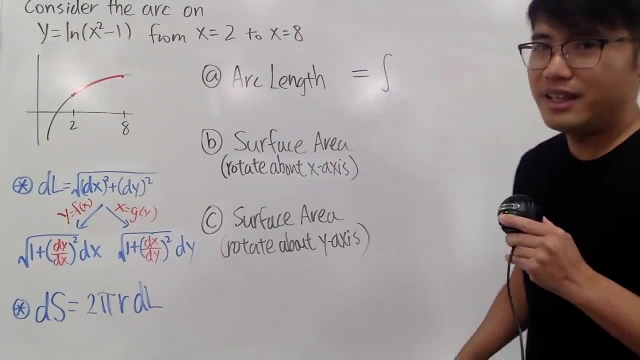 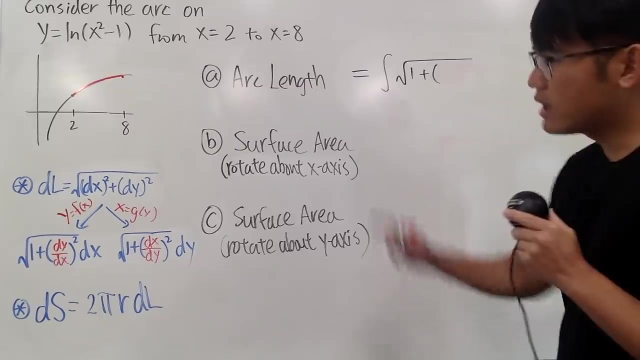 and we can end up with this side right. So here we have the square root, but let me put on the integral first, because this is just a small change in the r-length. You have to use integrals to add them up And we will have to put on the square root: 1 is 1 plus parentheses. Notice that. 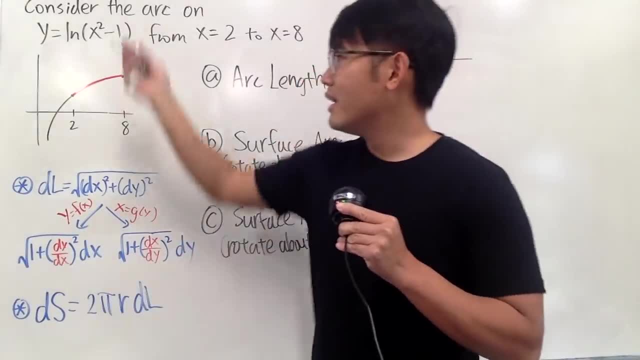 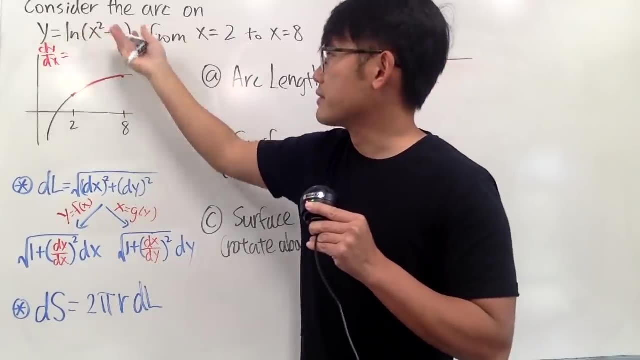 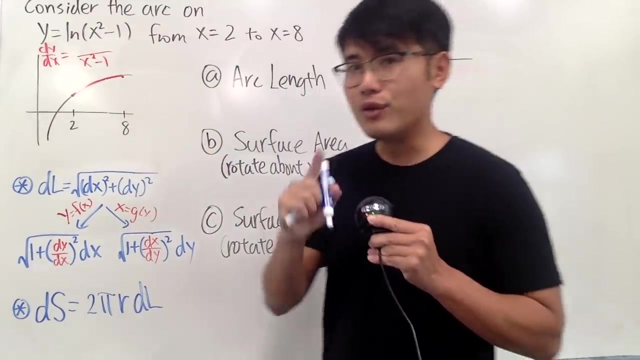 we have to get our first derivative. Let's look back to here. I will differentiate this: which we get dy, dx, and the derivative of natural of something is of course the derivative of the inside, which is 1 over the inside. So we have x squared minus 1 in the denominator, And don't. 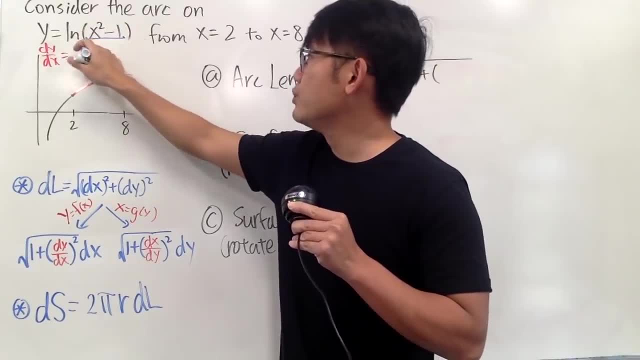 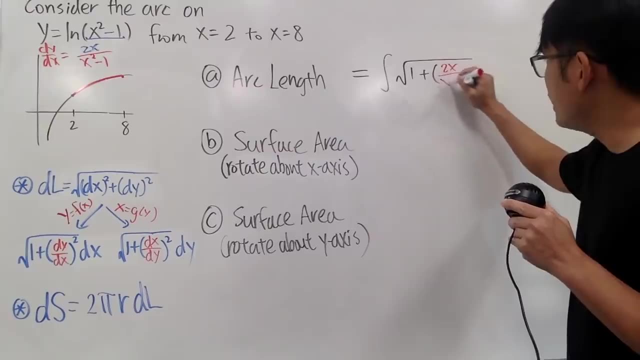 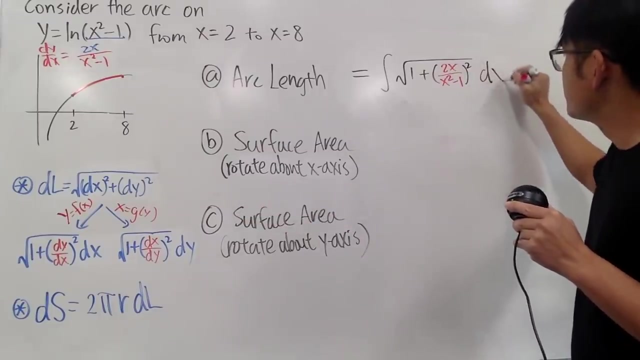 forget your chain rule. Multiply by the derivative of the inside, which you will get due to x, And we will just put that down right here. Let's write down: 2x over x, squared minus 1, and we square that And we also have to have the dx And, as you can see, because of the dx, we know that we have. 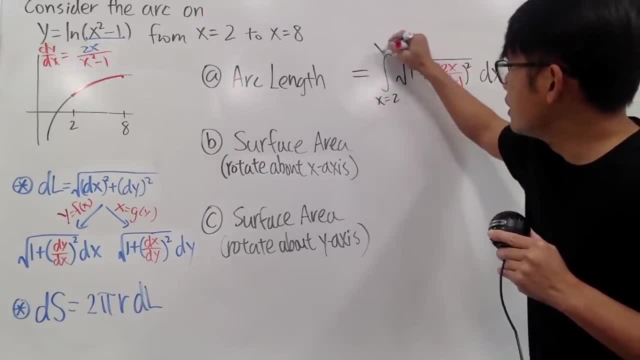 to set this up to be going from x squared minus 1 to x squared minus 1.. And we also have to have the dy dx, which is the derivative of the inside of the x squared minus 1.. And we will put that down right here And this will be our first derivative And if we can use that Cute- 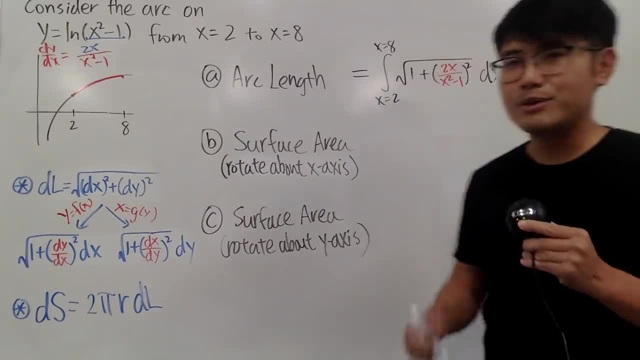 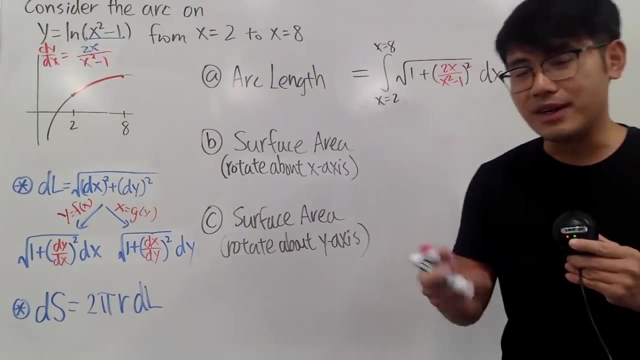 Autoparticle. we will get the accepted derivative of the laughing calculator And it will create a graph And it will have the same results as the previous one. So we are going to the whole surface, But the difference is that we will be calculating the graph of the surface. 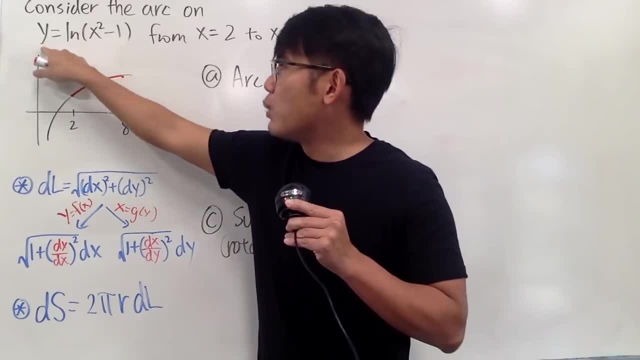 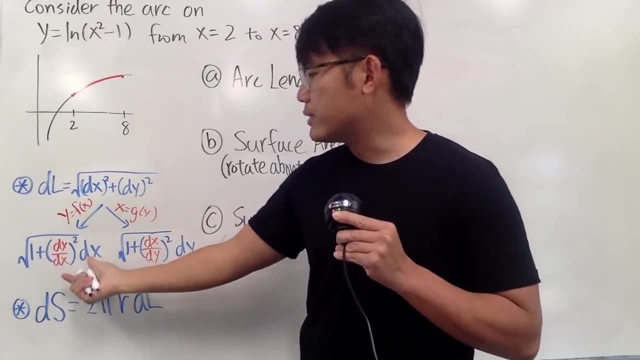 function of x or x as a function of y. In our case we have y as a function of x, so we'll use this version for it. Notice, I just have to factor out the dx squared and then do some algebra. 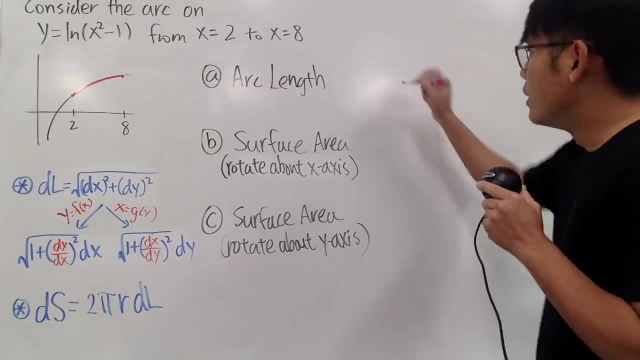 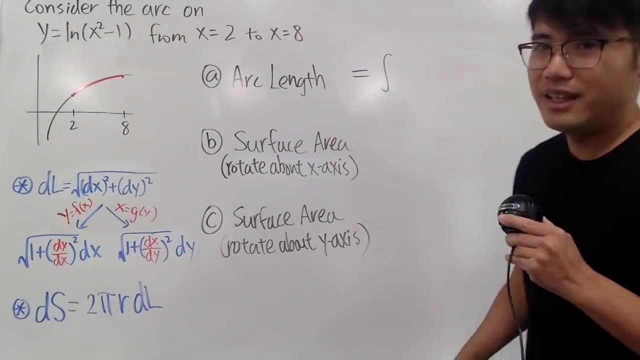 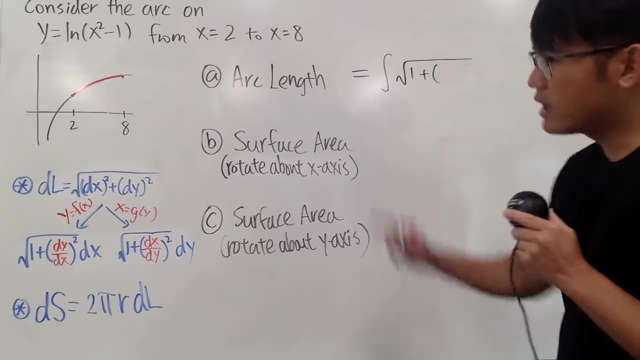 and we can end up with this side right. So here we have the square root, but let me put on the integral first, because this is just a small change in the r-length. You have to use integrals to add them up And we will have to put on the square root: 1 is 1, plus parentheses. Notice that. 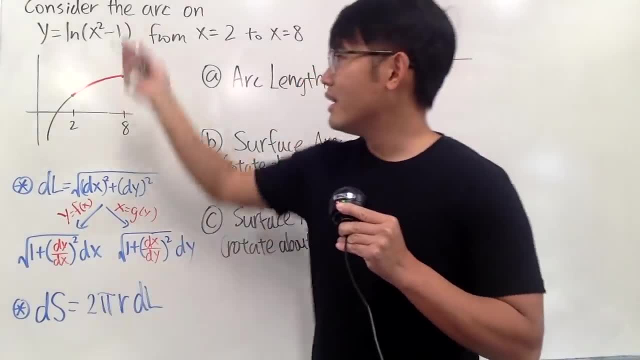 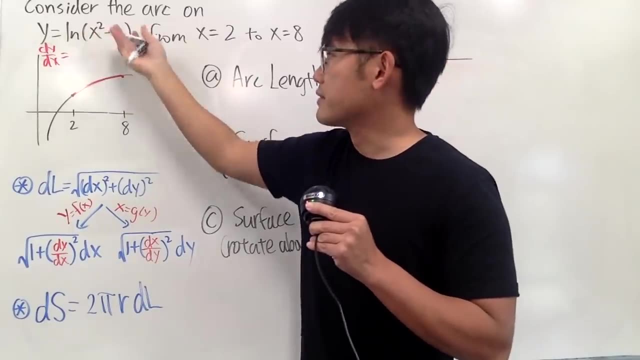 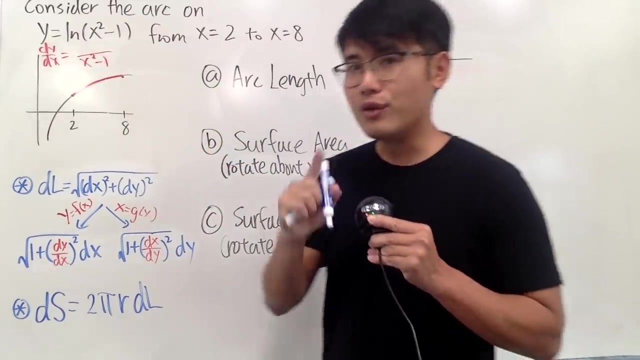 we have to get our first derivative. Let's look back to here. I will differentiate this: which we get dy dx, And the derivative of natural of something is of course the derivative of y dx, 1 over the inside. so we have x squared minus 1 in the denominator. And don't forget your. 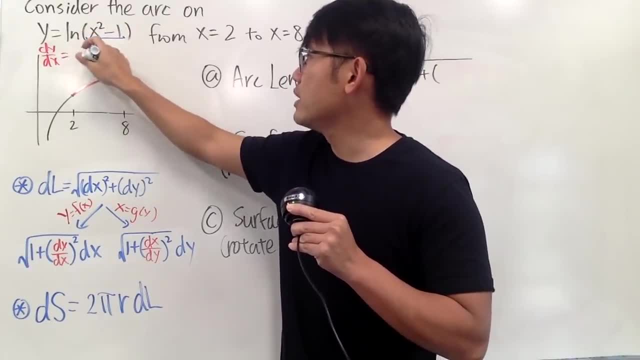 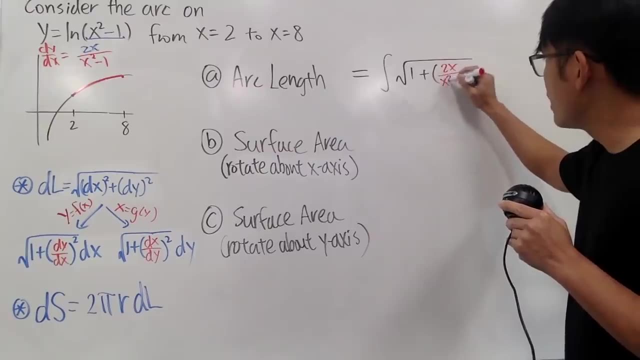 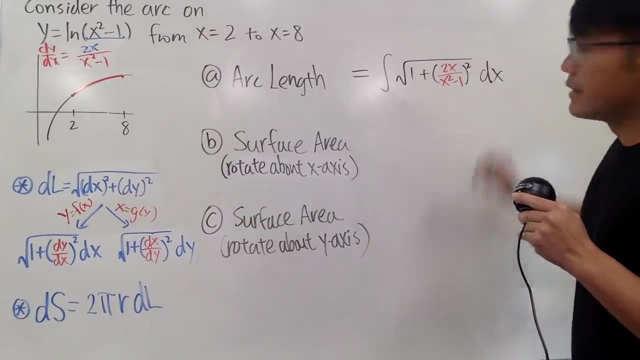 chain rule. Multiply by the derivative of the inside, which you will get due to x, And we will just put that down right here. Let's write down 2x over x squared minus 1, and we square that And we also have to have the dx And, as you can see, because of the dx, we know that we have to. set this up to be going from x squared minus 1 to x squared minus 1.. And we also have to have the dx, and we have to have the derivative of y squared minus 1, and we also have to have the x squared. minus 1, and we also have to have the derivative of x squared minus 1, and we also have to have the derivative of x squared minus 1.. And this should be equal to 2x plus 2x, that's 2x plus 2x squared. 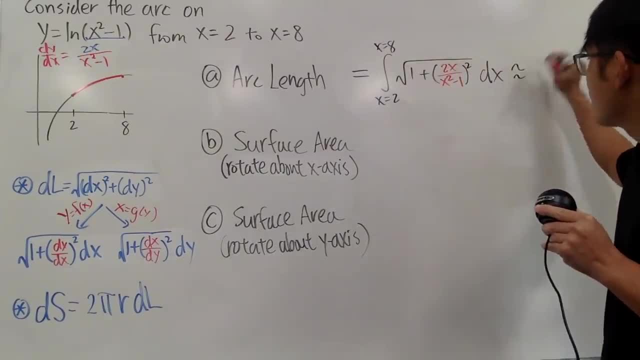 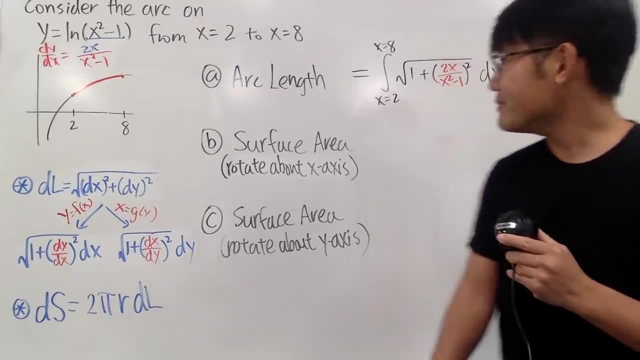 minus 1, equals 2x squared plus 2, up to 8.. And this, right here it's it Again. use your graphing calculator. Just practice how to use it, so you can do that later on on the exam, or so. 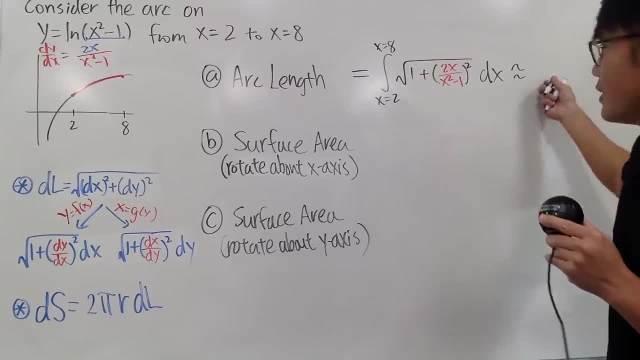 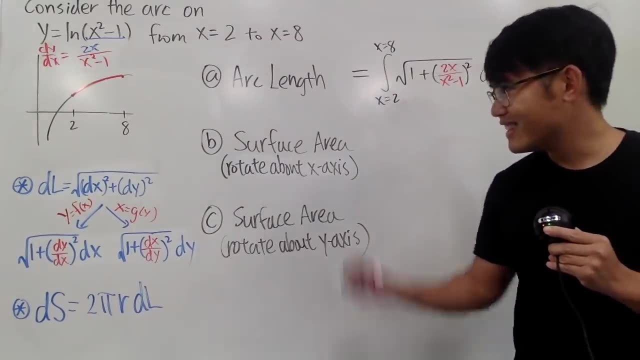 So maybe you guys can leave your comment down below and let us know what the answer to these questions are and whosoever can get it right or pinch your comment right. That would be cool, Okay. next, Surface area. Well, in this case the capital S stand for the surface area, so again, 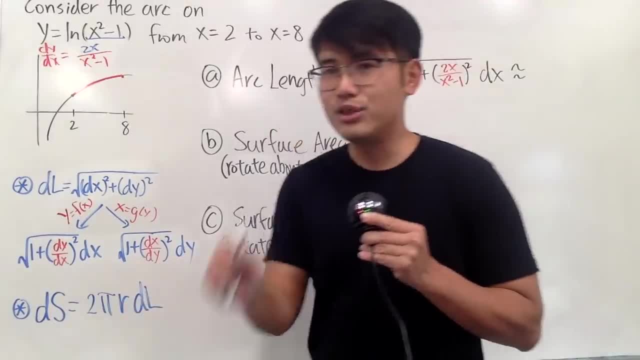 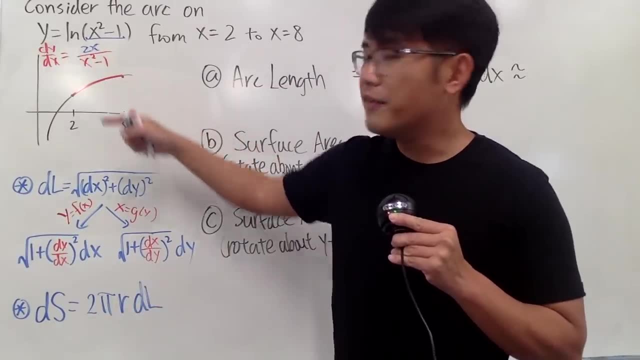 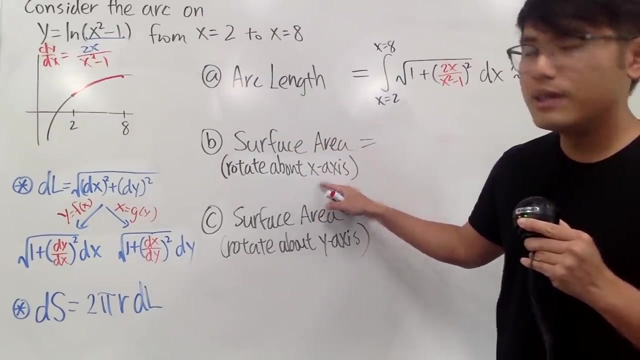 capital. S stands for the surface area and ds is just a small change amount in the surface area. Notice, the formula is 2 pi r. It's just like the circumference formula, right? And in our case here we are going to take the arc and rotate about the x-axis. So when you do that, the radius is the y. 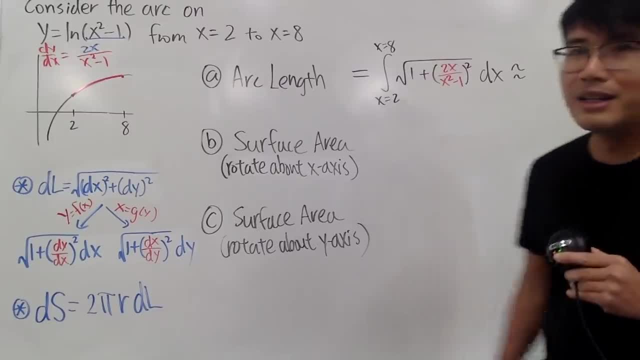 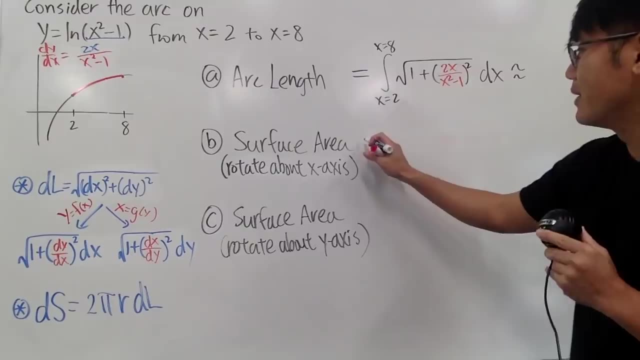 mark. So I'm going to write down again what this right here equals to 2, up to 8.. And this right here is it Again. use your graphing calculator. Just practice how to use it so you can do that later on in the example. So maybe you guys can leave a comment down below. 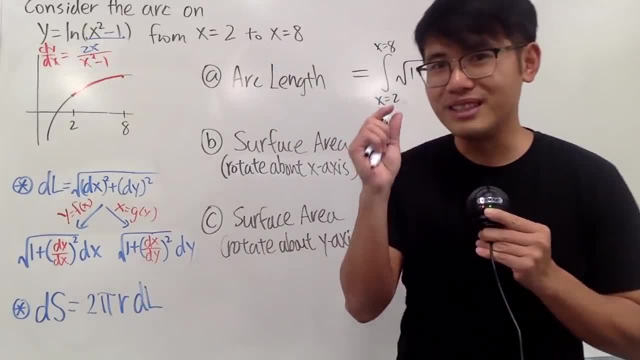 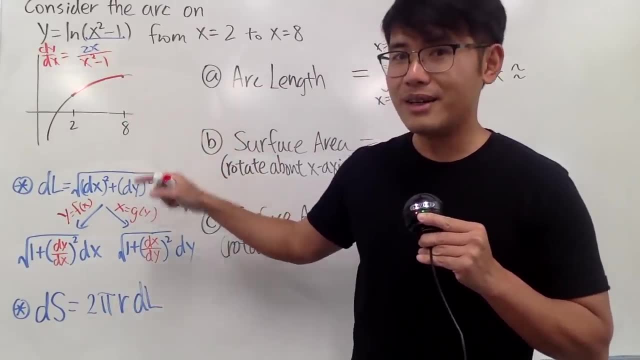 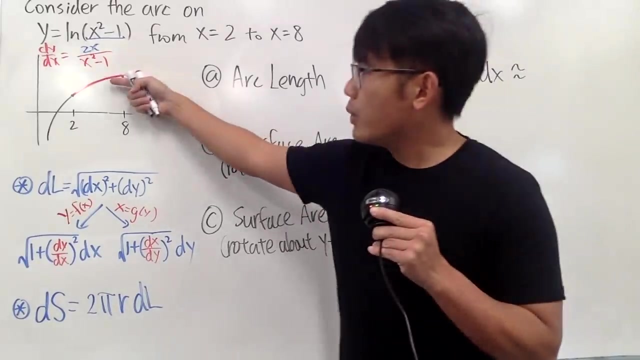 for the surface area, and ds is just a small change amount in the surface area. Notice, the formula is 2 pi r. It's just like the circumference formula, right? And in our case here we are going to take the arc and rotate about the x-axis. So when you do that, the 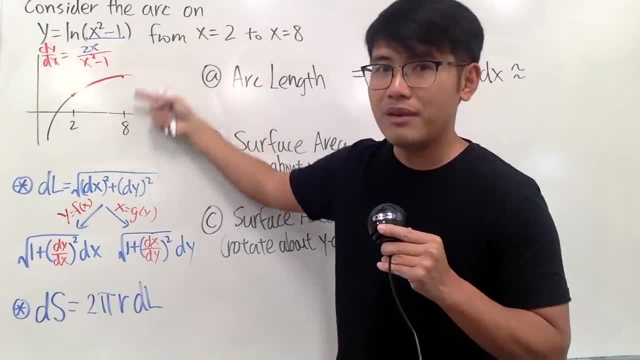 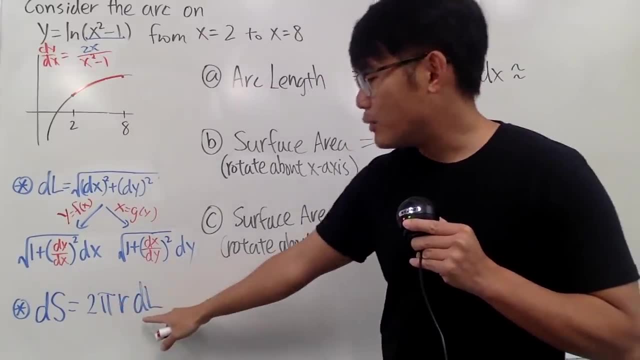 radius is the y-value. This right here is the y-value. when you have this rotation here And you take the circumference right, 2 pi r is the circumference formula, but you have to multiply by dl and the reason is because you have to make this slanted and then rotate. 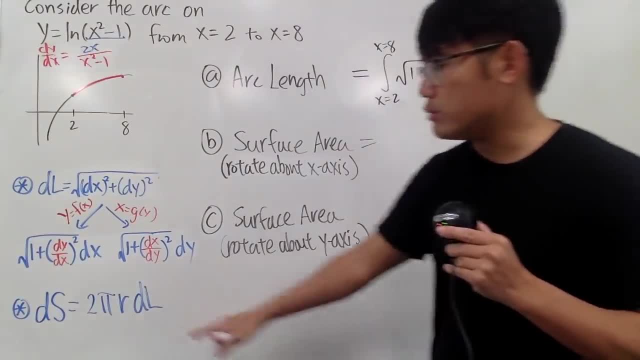 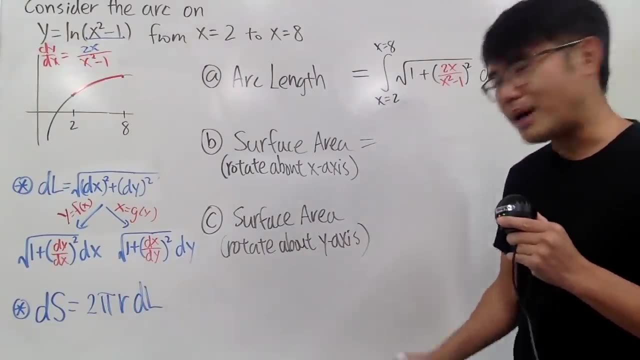 that And that's pretty much the quick explanation in a way that you can remember this formula nicely, and you guys can see my other videos for a detailed explanation for why that formula is true. But anyway, enough talking, here we go. 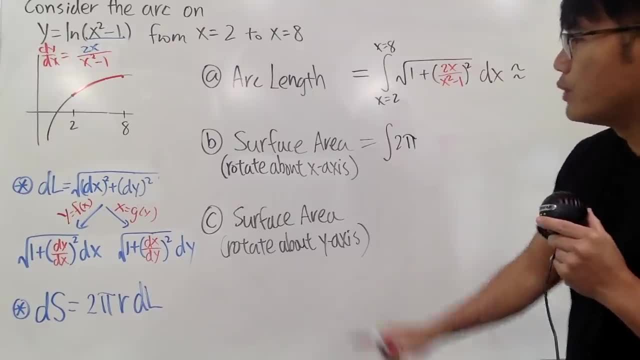 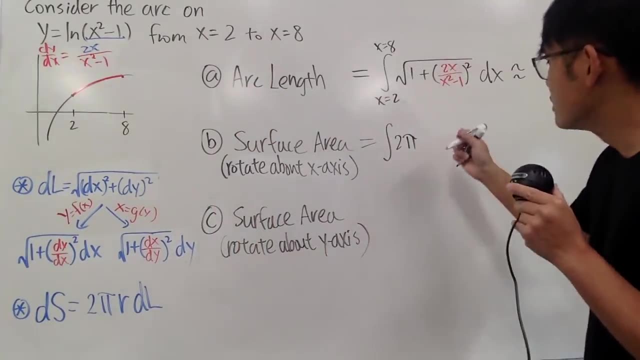 We have to have the integral, of course, 2 pi. when we rotate about the x-axis, the radius is: is again the vertical distance, which is the y value. So let me put down the y and then we put down the dl, of course. 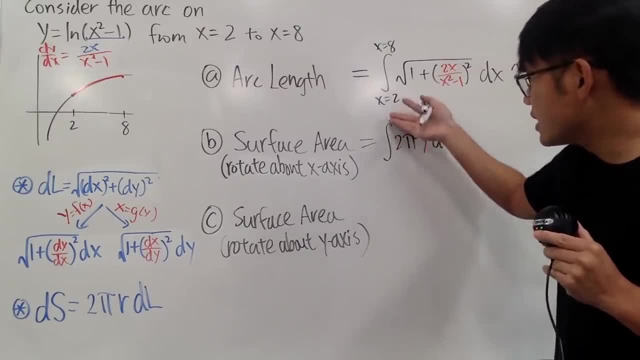 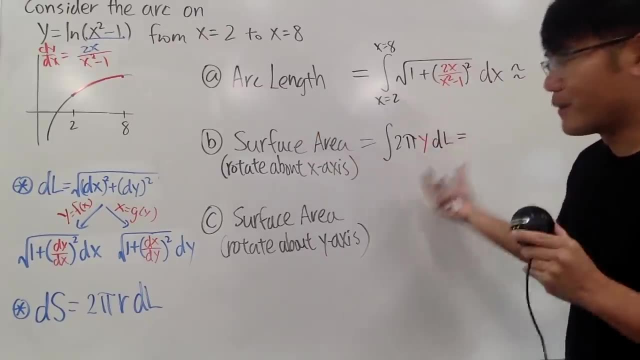 And you see that we have to have the dl here. I cannot set up the limits of integration yet. Well, we have to look back to first part, And if you are doing this question like from scratch by itself, then you have to look back. 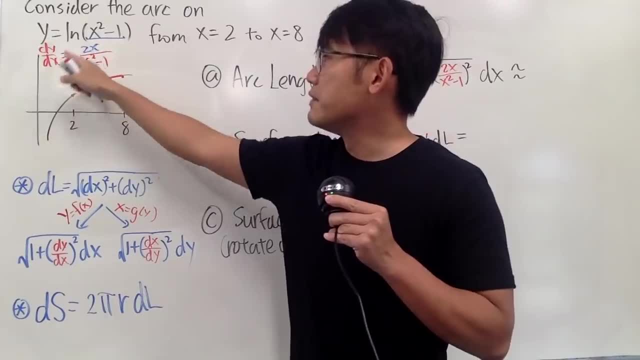 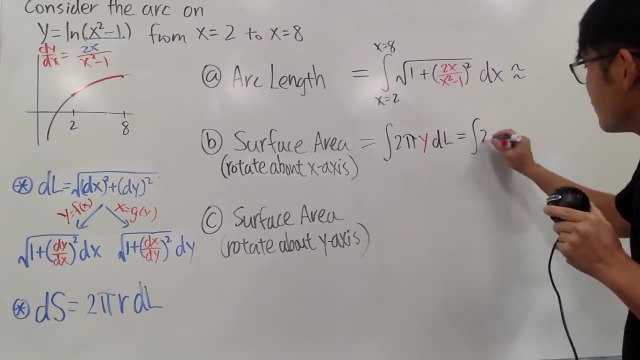 to see what kind of function you have. Because we have y as a function of x, we will have to use this version for the dl right. So let's see Integral. we have two pi. it's still two pi. 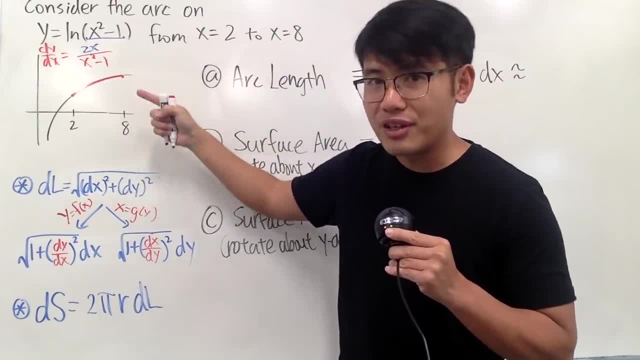 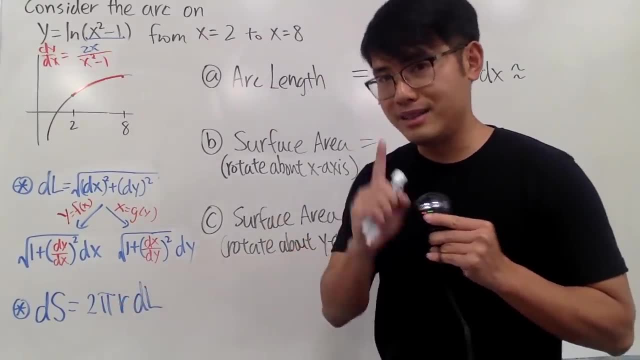 value right. This right here is the y value. when you have this rotation here And you take the circumference right, 2 pi r is the circumference formula, but you have to multiply by dl, And the reason is because you have to make this slanted and then rotate that And that's pretty much the 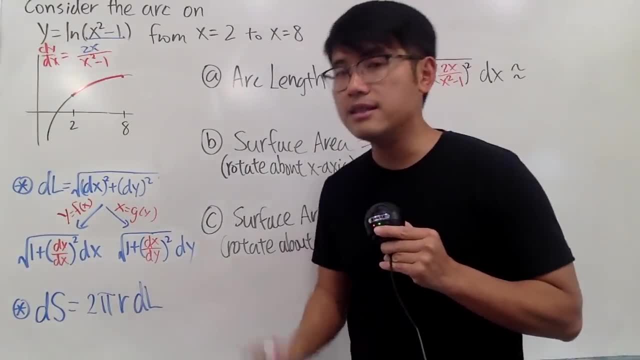 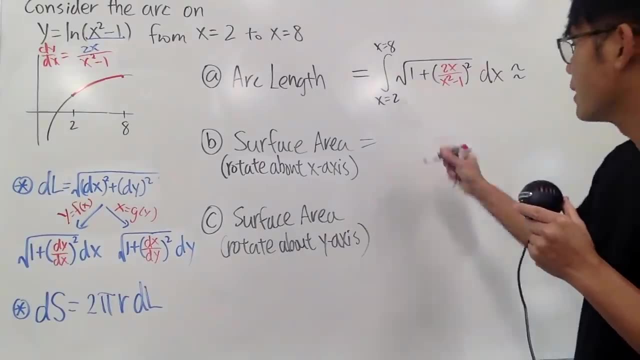 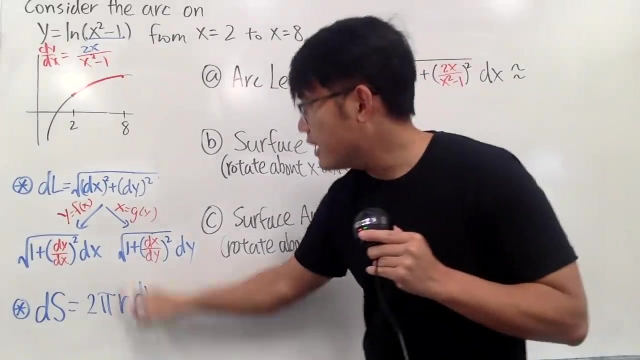 quick explanation in a way that you can remember this formula nicely, and you guys can see my other videos for a detailed explanation for why that formula is true. By the way, enough talking, here we go. We have to have the integral, of course, 2 pi. When we rotate about the x-axis, the radius is again. 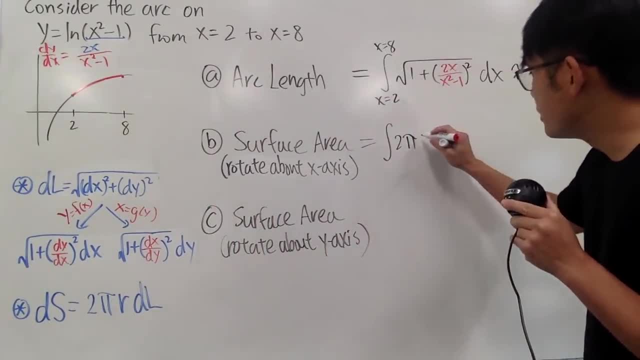 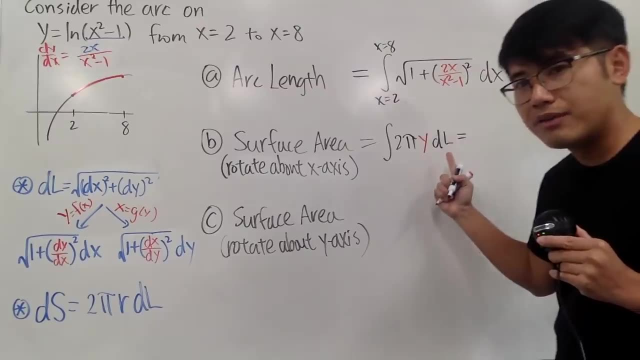 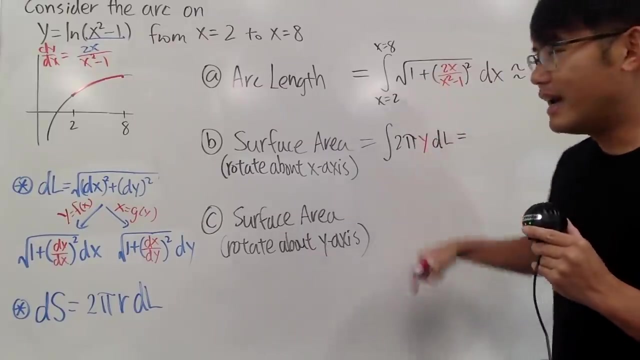 vertical distance, which is the y value. So let me put down the y and then we put down the dl. of course, And you see that we have to have the dl here- I cannot set up the limit of integration yet. Well, we have to look back to first part And if you are doing this question, 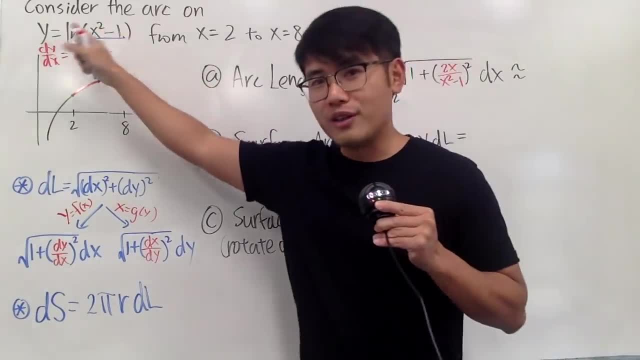 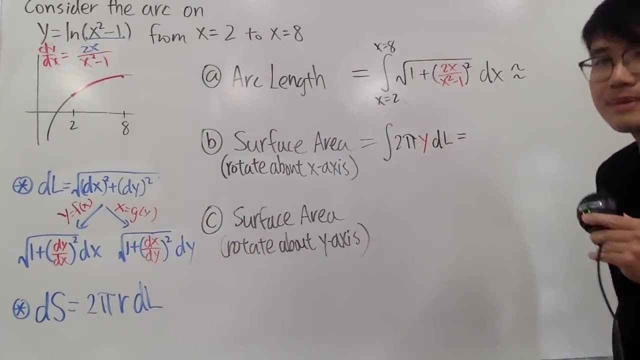 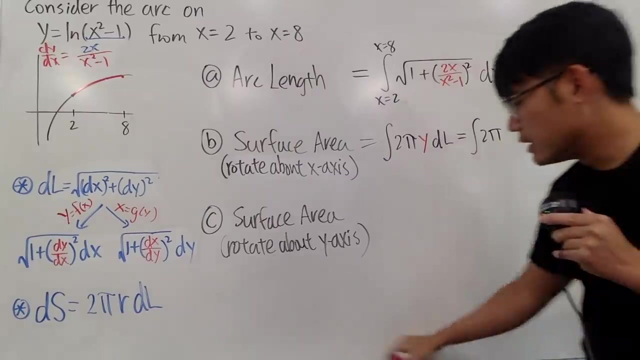 from scratch by yourself, then you have to look back to see what kind of function you have, Because we have y as a function of x. we will have to use this version for the dl, right? So let's see Integral. we have 2 pi. it's still 2 pi. We have this y, But again for the dl. 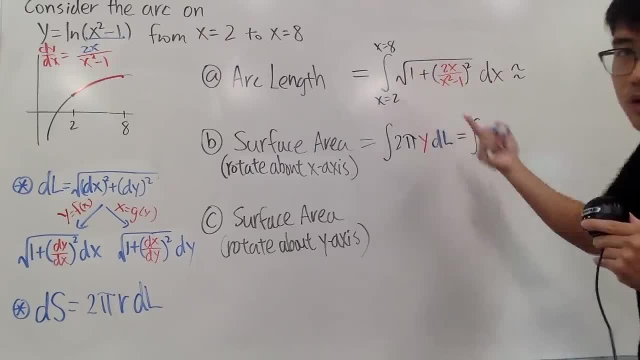 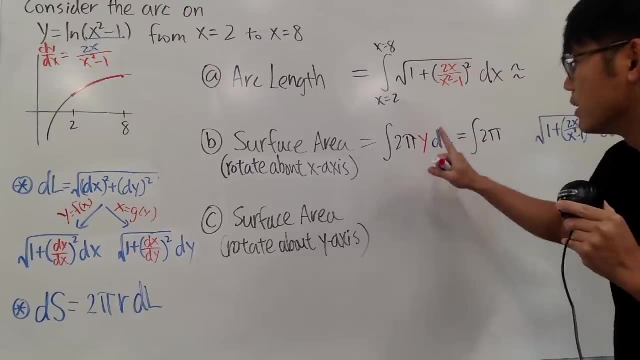 it's pretty much the first part, just the inside, without the integration of course. So let me put that down right here. And now here's the dl. Earlier, we talked about it. When we rotate about the x-axis, the radius is y. But now we are in. 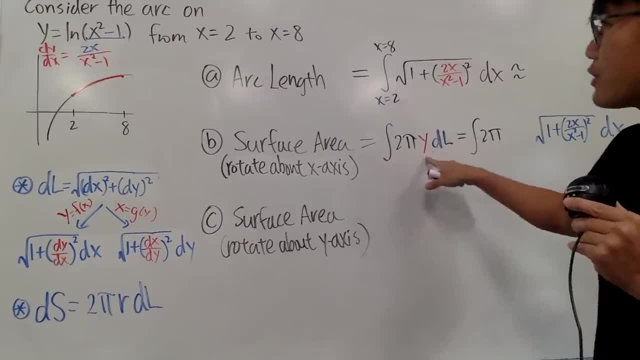 the x-world. So we are in the x-world. So when we rotate about the x-axis, the radius is y, But now we are in the x-world. We have to actually look back to what y is in terms of x. So we have to actually write this. 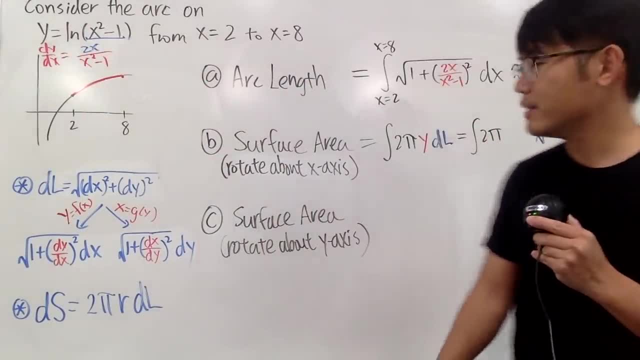 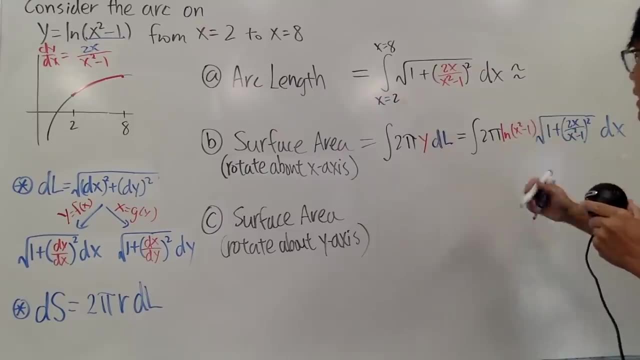 down. because, again, y is not invited in the x-world. So write down this y as the natural log of x squared minus 1.. Like this. And because we are in the x-world, we are going to go from x equals 2 to 8, like that. So this, right, here is again the setup, and you guys just 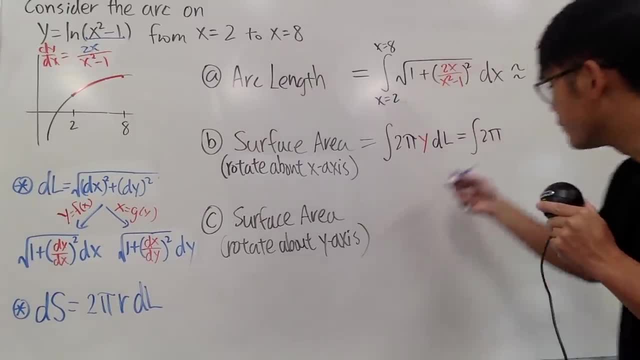 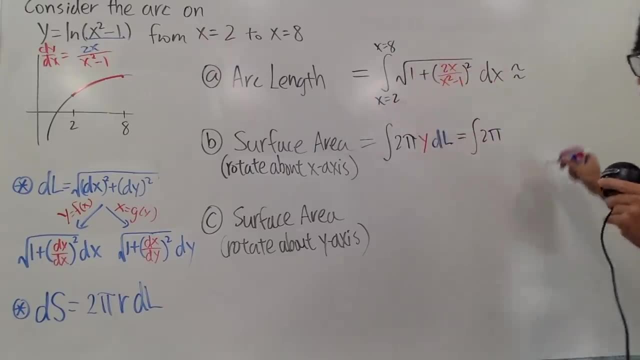 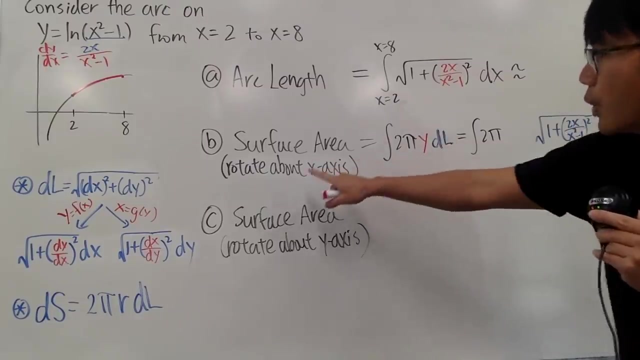 We have this y, But again for the dl, it's pretty much the first part, just the inside, without integration of course. So let me put that down right here And now. here's the dl Earlier, we talked about it. 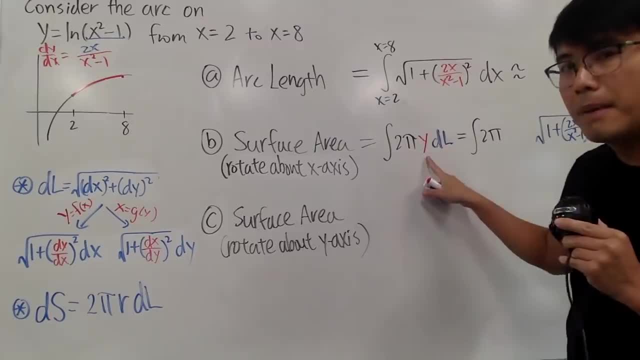 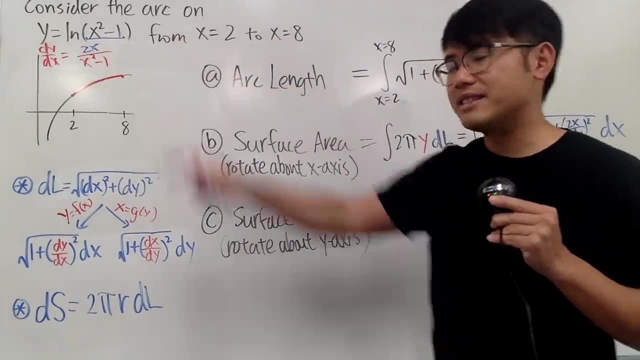 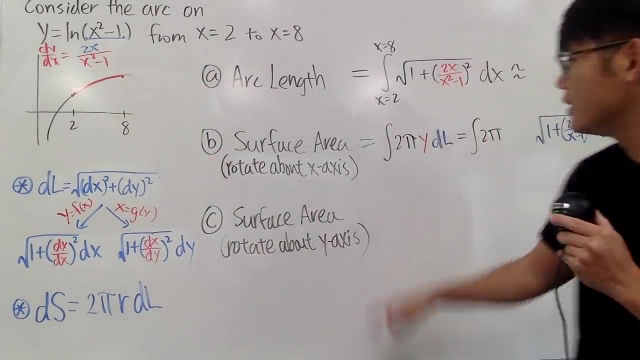 When we rotate about the x-axis, the radius is y, But now we are in the x world. So we have to actually look back to what y is in terms of x. So we have to actually write this down Because, again, y is not invited in the x world. 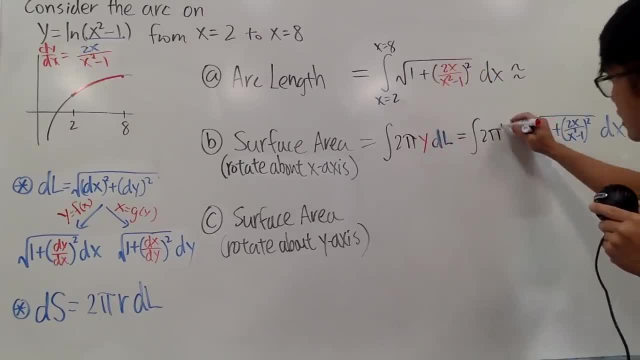 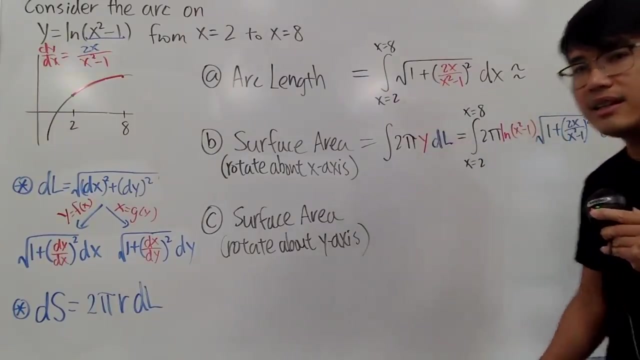 So write down this y as the natural log of x squared minus one, like this. And because we are in the x world, we are going to go from x equals two to eight, like that. So this right here is again the setup. 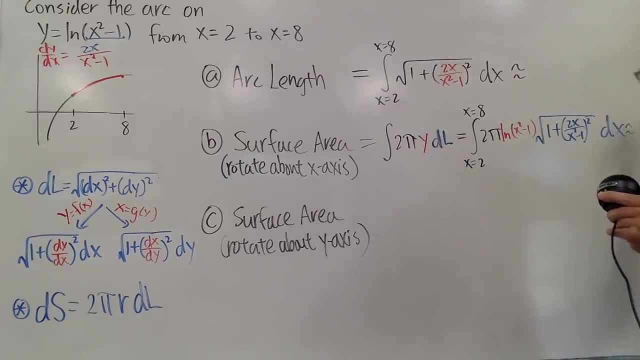 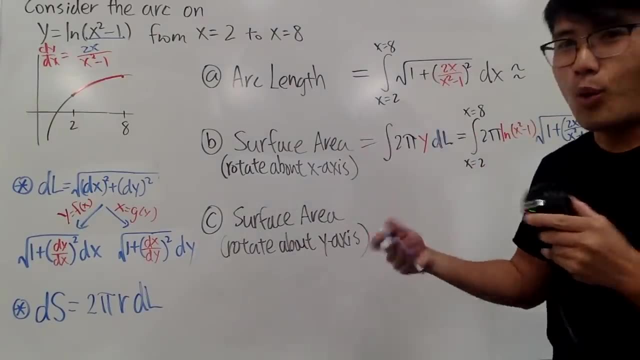 And you guys just use the calculator to do the approximation for us, So that'll be cool. Okay, All right, okay, So it's okay anyway To find the surface area. if you take the arc rotate about the y-axis. 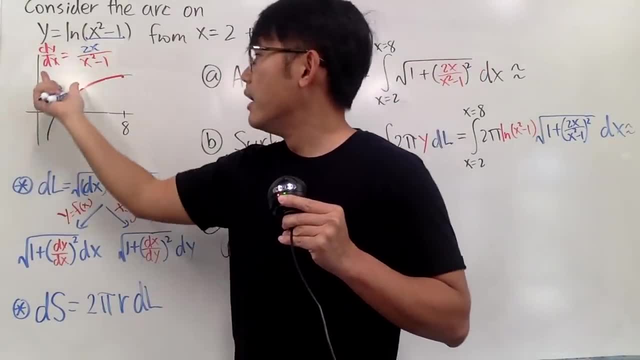 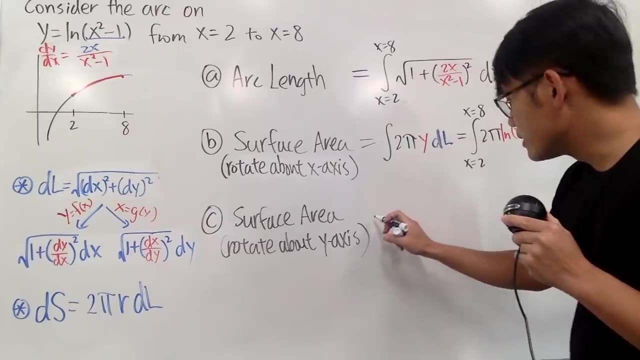 the only thing different is that when you do it this way, the radius is horizontal, So it's actually the x values. now, right? So I will write this down right here for you guys. This right here is equal to: 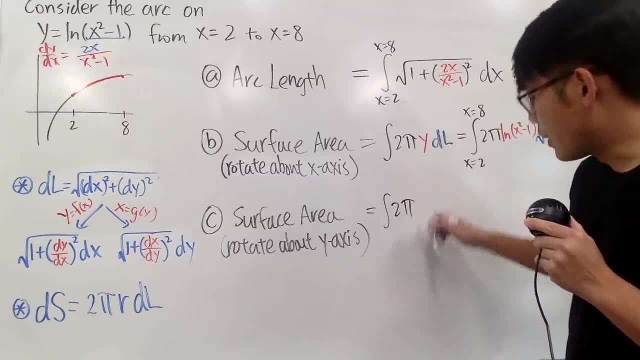 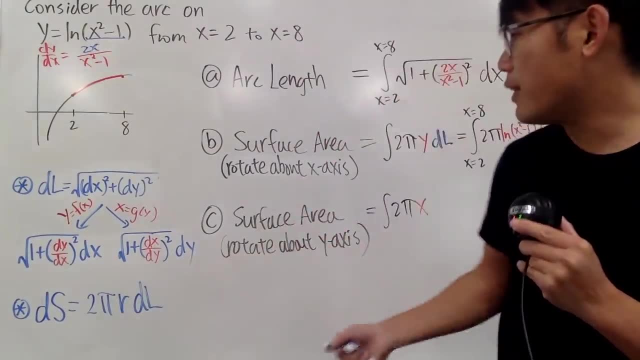 the integral two pi, and again, in our case, here it's x, right? So this part, the radius, you have to think about it depending on how you rotate, And the dl is still dl, so I will just put that down. 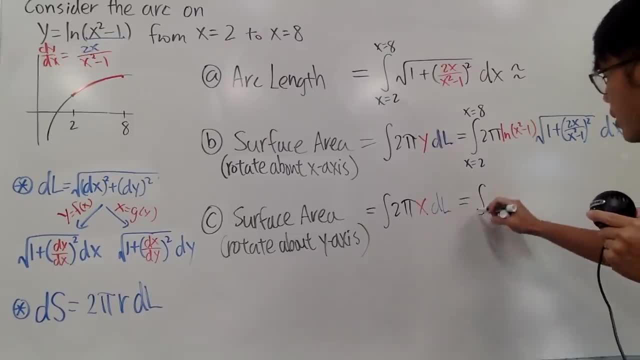 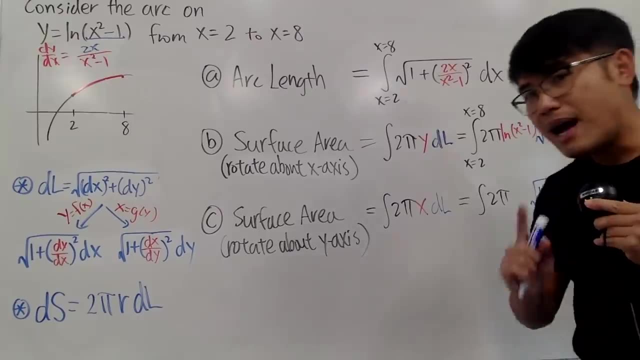 And you'll see, this is actually really nice because you can just have the integral two pi. Well, let me write down the dl for you guys. first, which is still this part, But because we are in the x world, this part, this part. 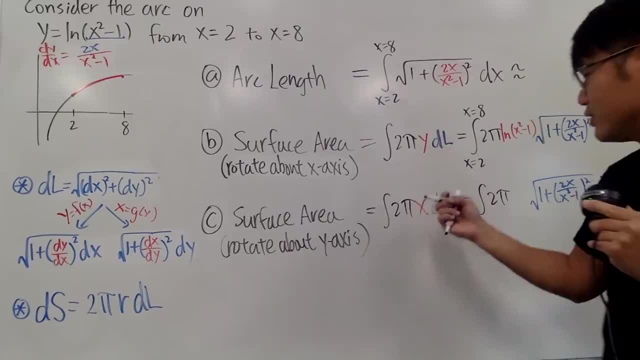 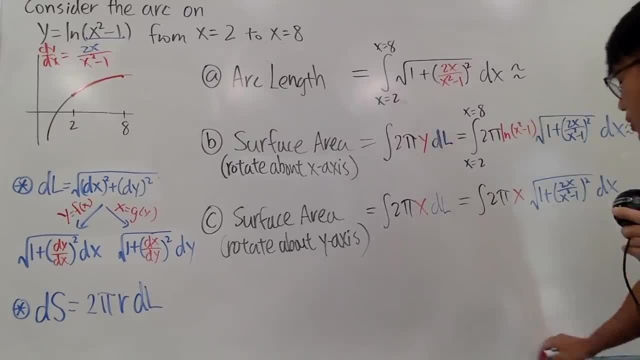 You can just go ahead and put down the x, so that will be your legitimate integral. And, of course, don't ever forget your limit of integration. in the x world we go from two, two, eight. So that's it. 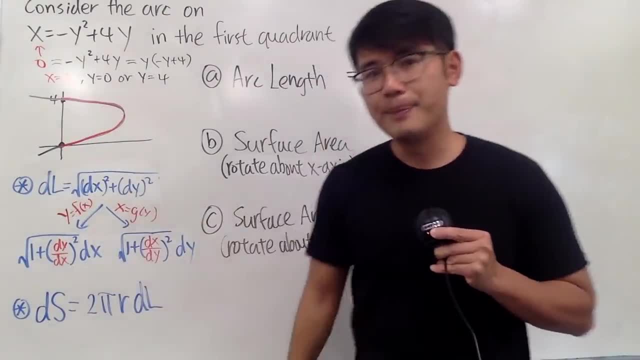 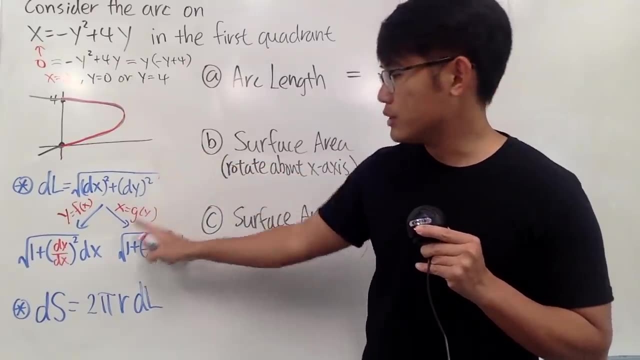 Here we go, Let's find the r length first versions. this time we will have to use this version because we have given x as a function of y, so use this version for it. so let's go ahead, put on the integral sign, add up all the little. 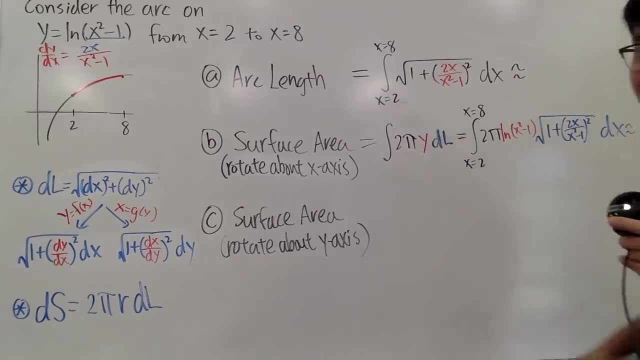 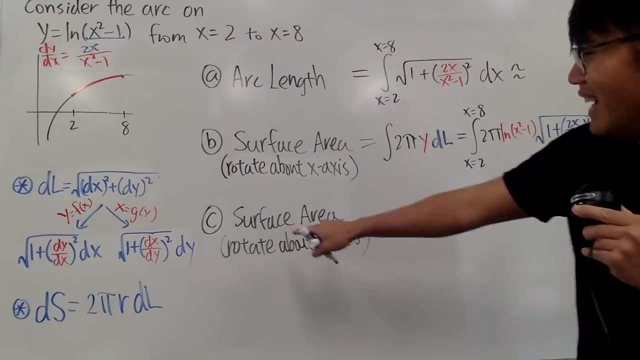 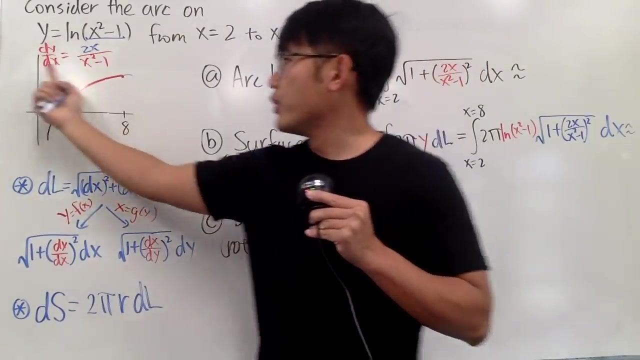 use the calculator to do the approximation for us. So that would be cool. Okay, All right, okay, so it's okay anyway To find the surface area. if you take the arc rotate about the y-axis. the only thing different is that. 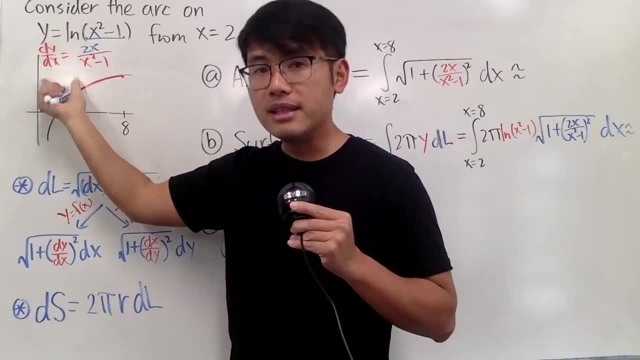 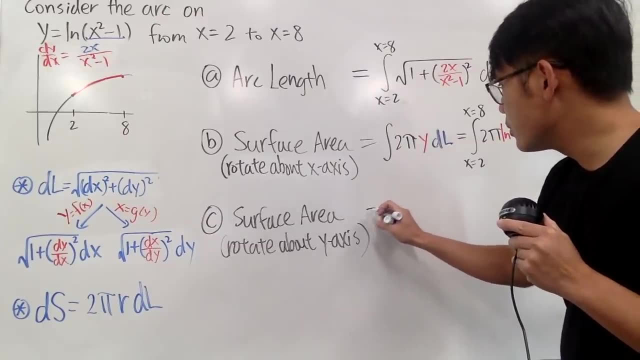 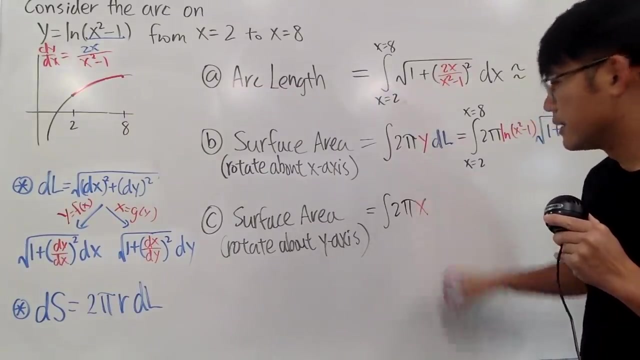 when you do it this way, the radius is horizontal, So it's actually the x values now, right? So I will write this down right here for you guys. This right here is equal to the integral two pi, and again, in our case, here it's x, right? 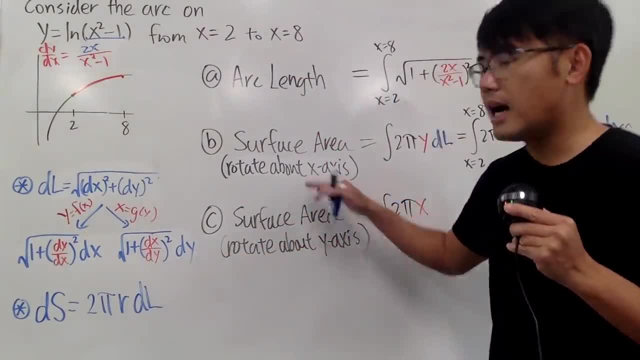 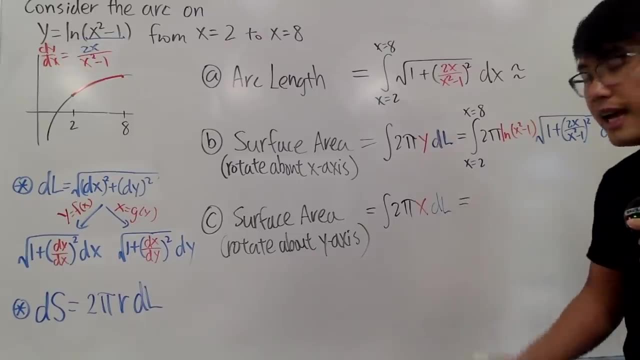 So this part, the radius, you have to think about it depending on how you rotate, And the dl is still dl. so I will just put that down And you'll see this is actually really nice because you can just have the integral two pi. 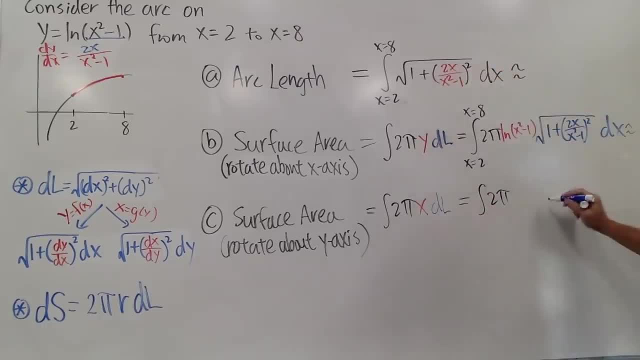 Well, let me write down the dl for you guys first, which is still this part. but because we are in the x-axis in the x-world, this x is totally fine. You can just go ahead and put down the x, So that will be your legitimate integral. 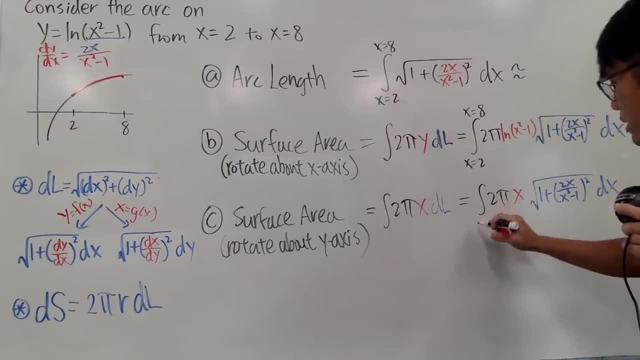 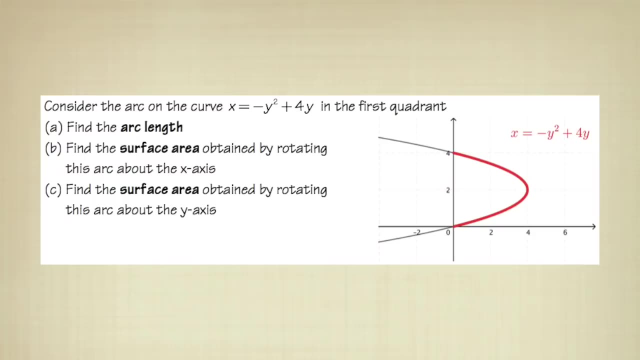 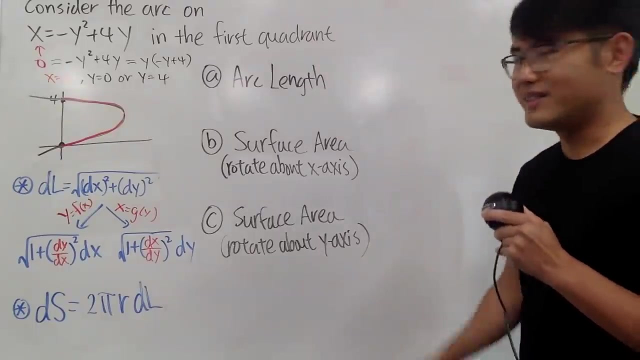 And, of course, don't ever forget your limit of integration. In the x-world we go from two to eight. So that's it. Here we go. let's find the arc lengths first. Well, well, So we have two versions. 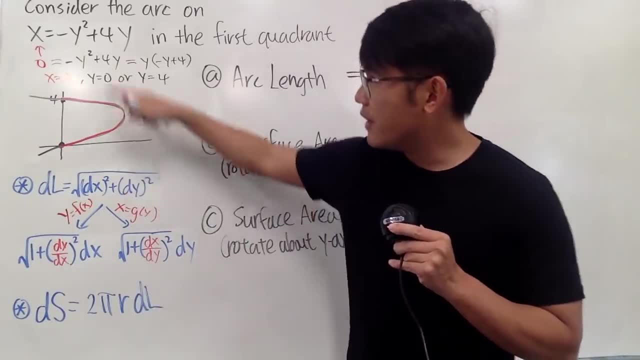 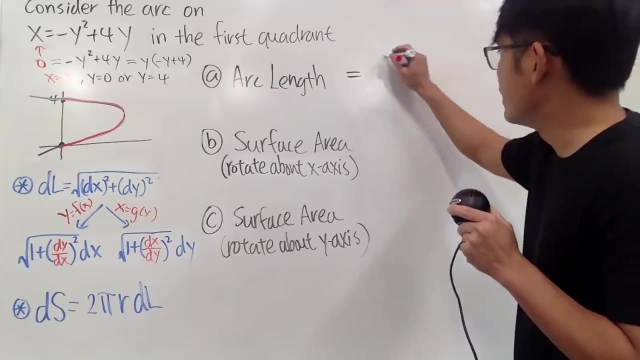 This time we will have to use this version because we have given x as the function of y, So use this version for it. So let's go ahead and put down the integral sign. add up all the little dls, right? 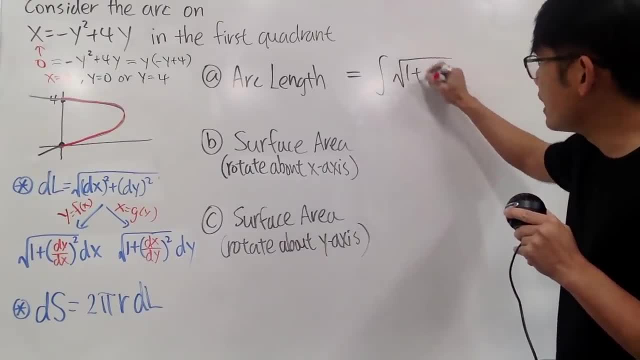 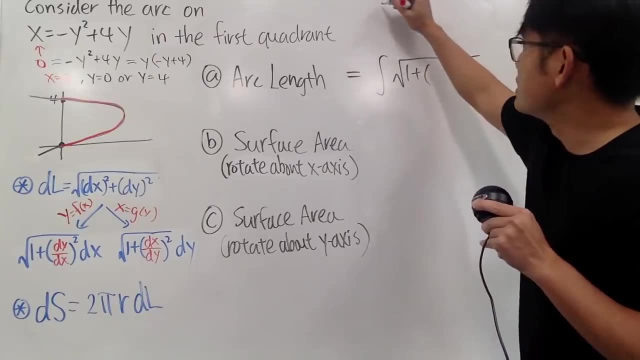 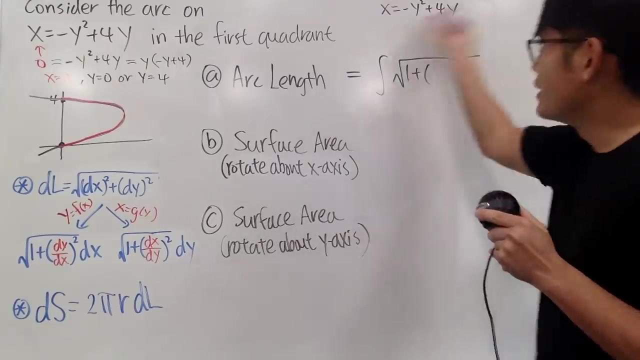 and we have the integral of the square root of one, plus parentheses. Okay, I need a dxdy now. Well, let me write it down right here for you guys. We know x is equal to y squared plus 4y dx, dy is. just look at this equation and do your usual derivative. 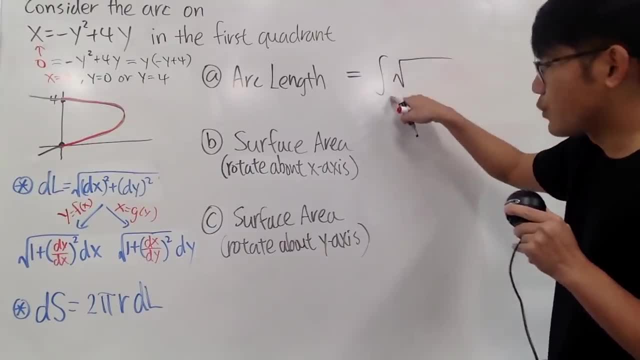 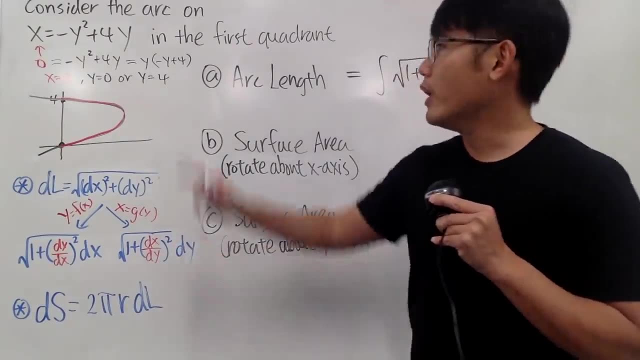 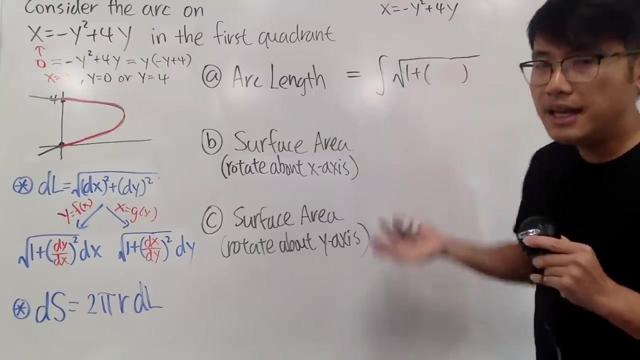 dl's right and we have the integral of the square root of one, plus parentheses. okay, i need a dx dy now. well, let me write it down right here for you guys. we know x is equal to negative, y squared plus 4y, dx dy is. just look at this equation and do your usual derivative. 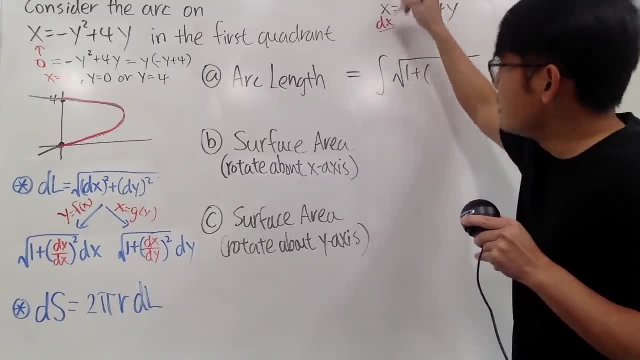 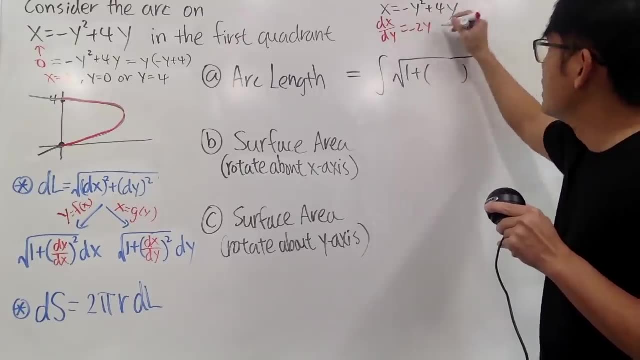 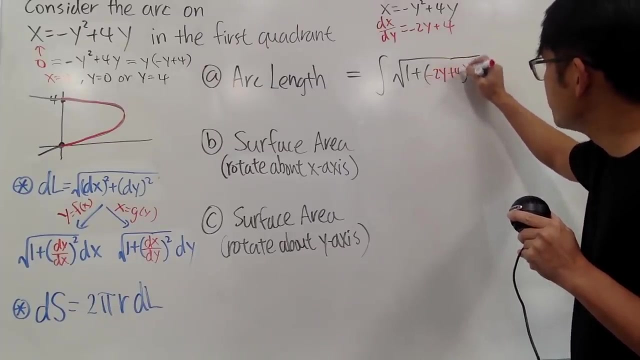 but you treat this as your dependent variable now and y as your independent variable and just go ahead and do it the usual way. you get negative 2y plus 4, okay, and you put this right here inside negative 2y plus 4, and don't forget the little square. 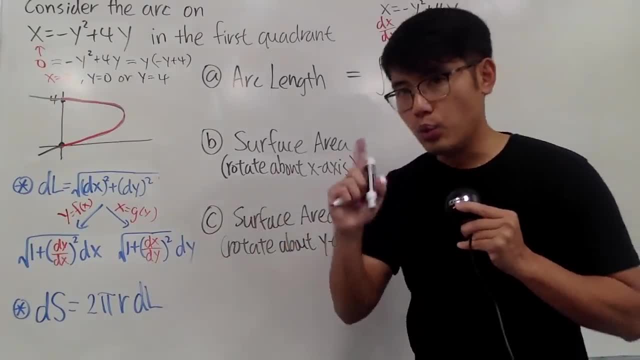 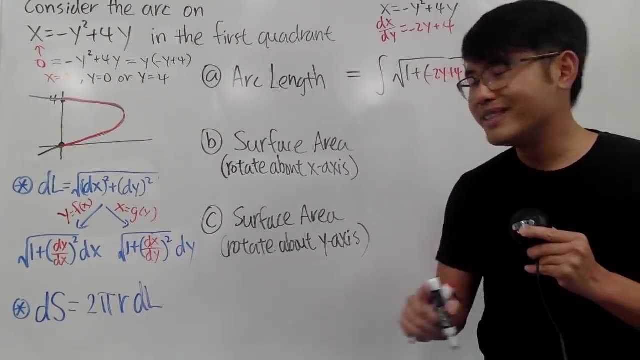 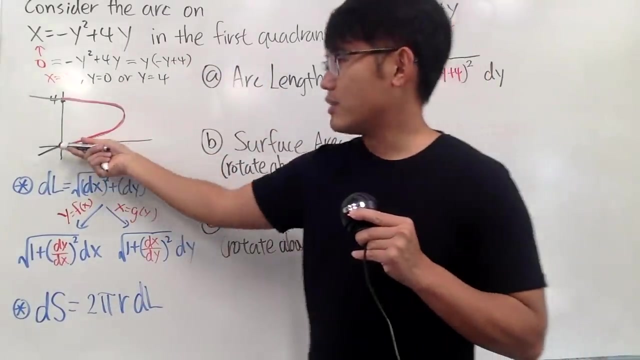 right here. And in this case we are in the y world, So put down the dy here. and because we are in the y world, we have to look for the y values going from where to where, And we did it Starting from here up to here, from zero to four. 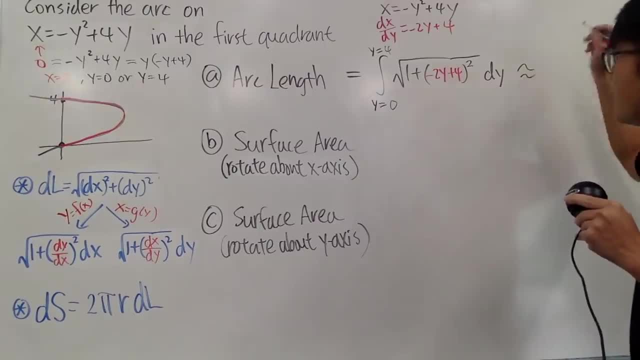 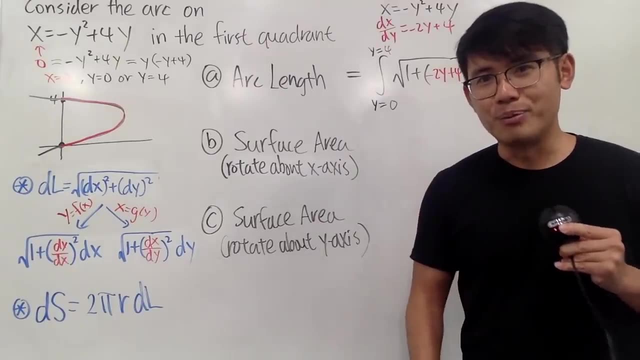 So that's nice and we are done And, just like the last video, go ahead, use your TI-T3 or TI-T4,, compute it and leave a comment down below and you can be the hero. People will like your comments. 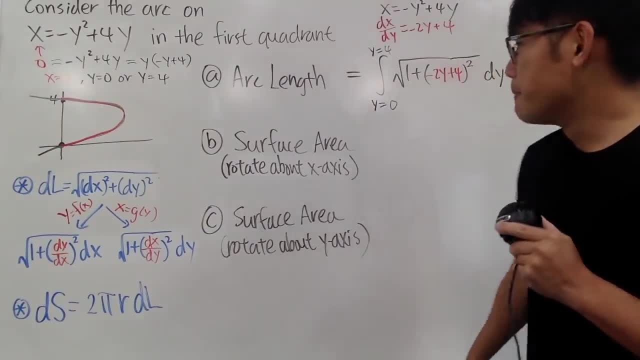 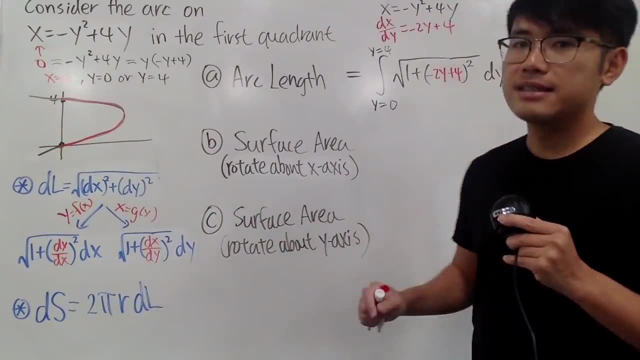 and you'll feel proud of yourself, right? So do that, Okay. next we will talk about the surface area. and now here's the deal. We will take this arc and rotate about the x-axis and, yes, you will see that. 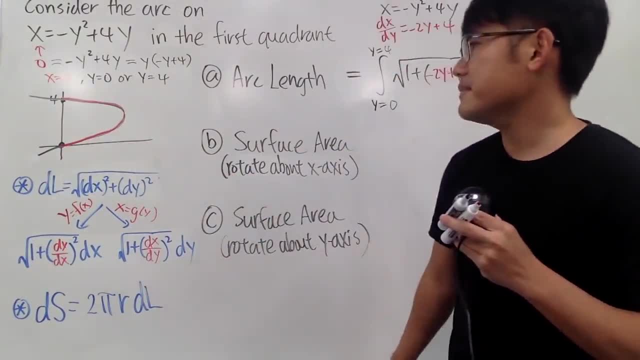 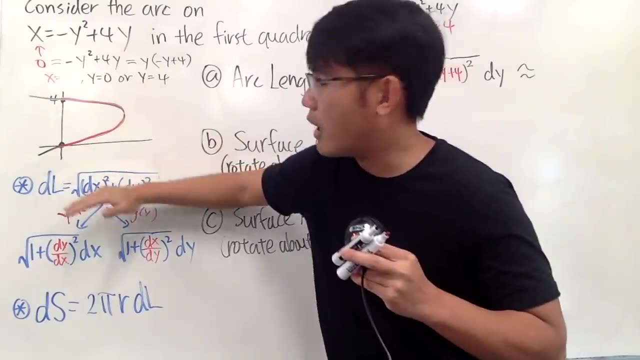 there's like one little part is missing. but the deal is that we look for the surface area. so it's like this: this kind of shape, And then the surface area. you have the outer part and then you also have the inner part. 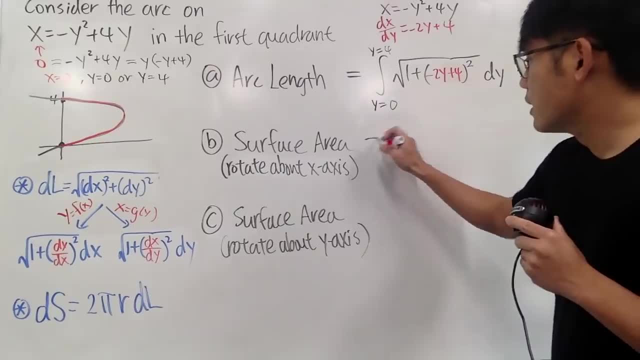 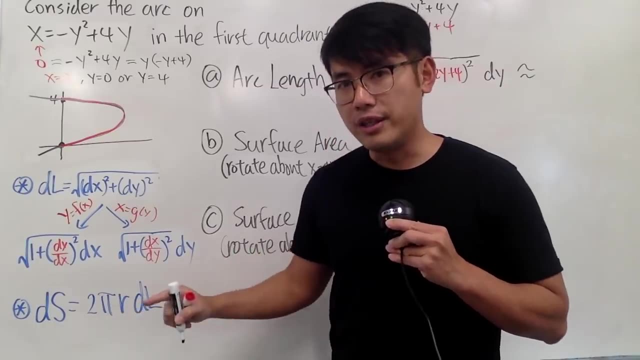 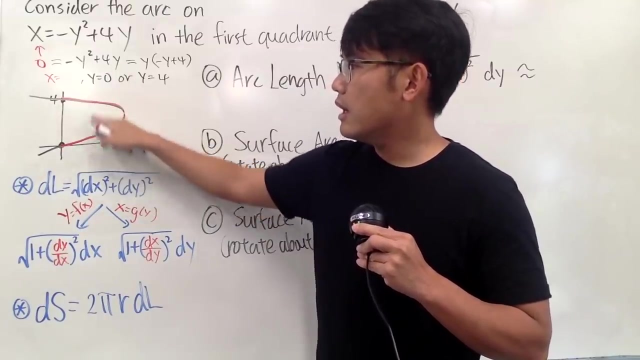 right, But anyway, for the surface area. first we have to look at the ds Formalize 2 pi r times. dl, r is the radius. Well, if you have a point right here, for example, the radius is just going to be the y-value. 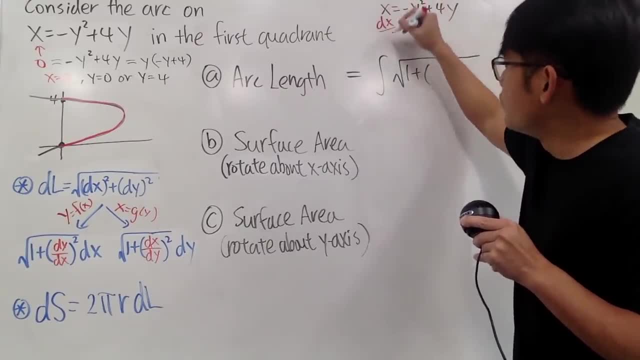 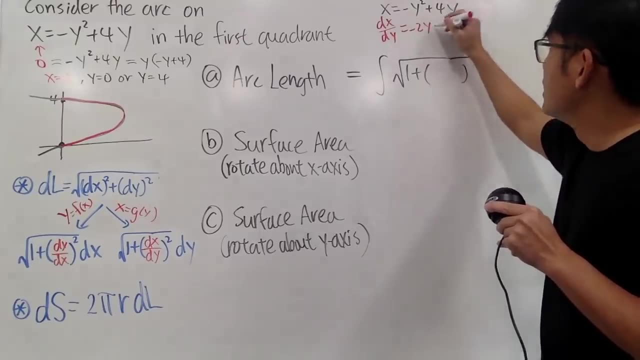 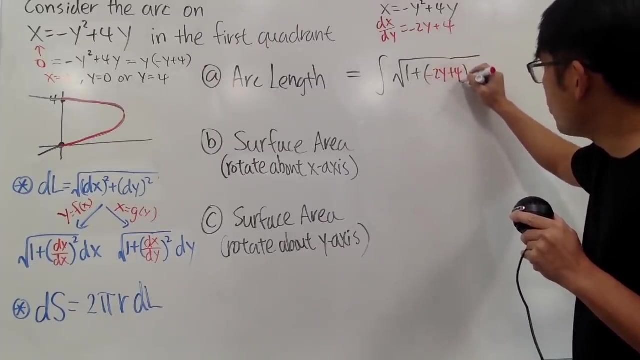 but you treat this as your dependent variable now and y as your independent variable and just go ahead and do it the usual way. You get negative 2y plus 4,, okay, And you put this right here inside Negative 2y plus 4, and don't forget the little square right here And in this. 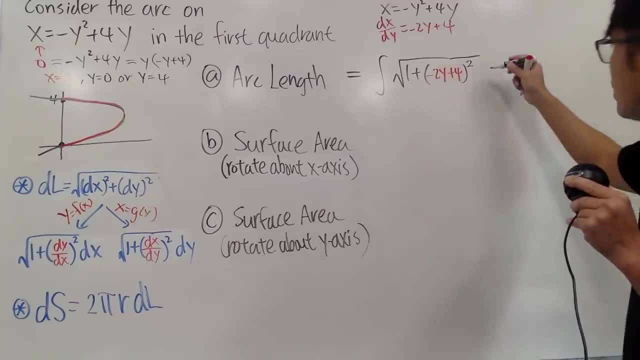 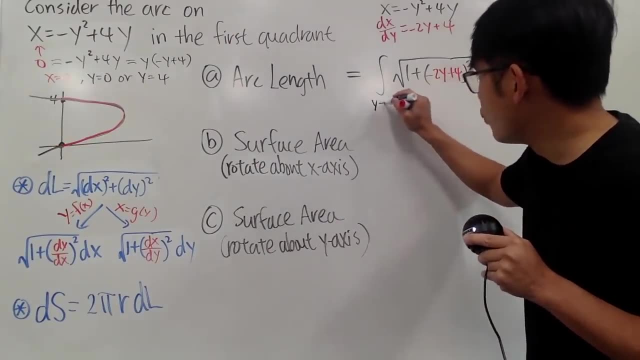 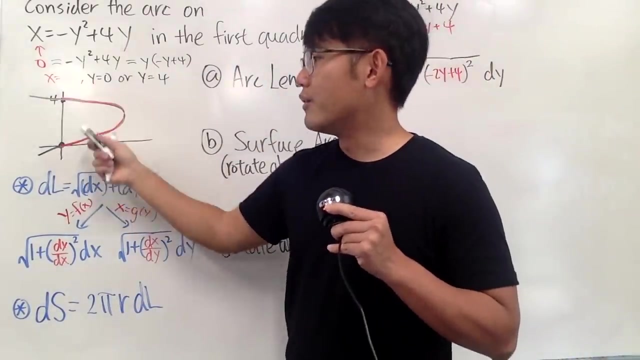 case. we are in the y world, So put down the dy here. and because we are in the y world, we have to look for the y values going from where to where, And we did it Starting from here up to here, from 0 to 4.. So that's nice and we are done. 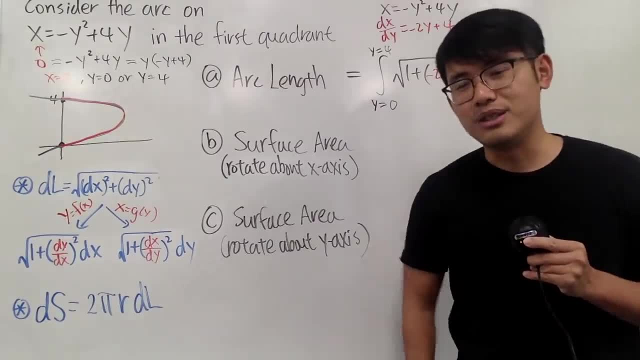 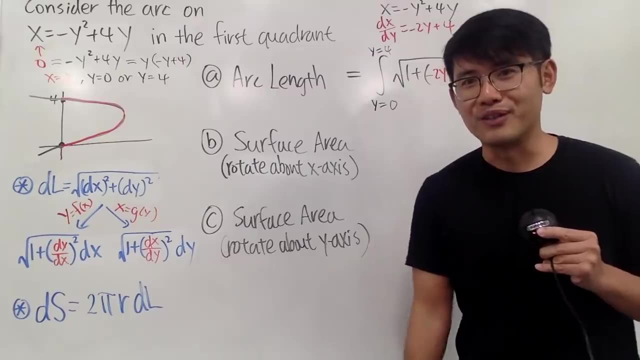 And we are done. And, just like the last video, go ahead, use your TIT3 or TIT4, compute it and leave a comment down below and you can be the hero. People will like your comments and you'll feel proud of. 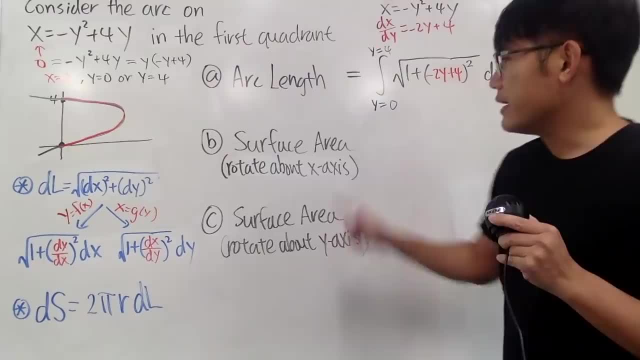 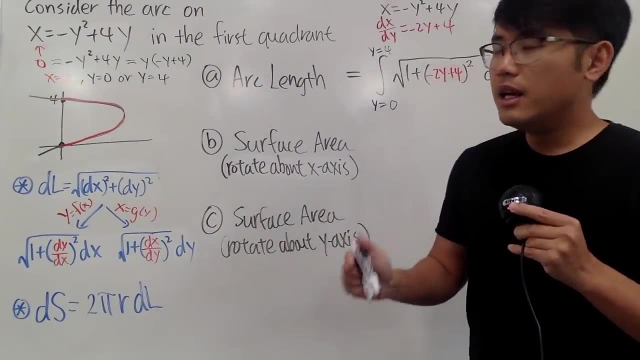 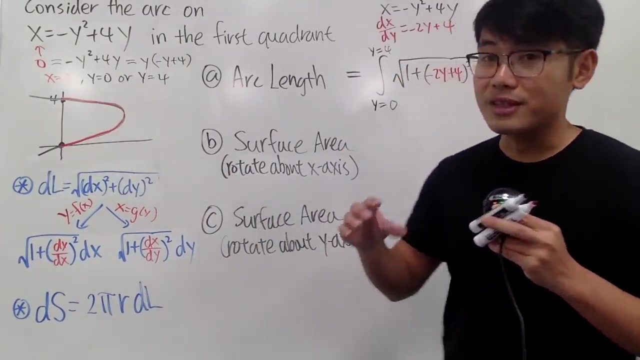 yourself right, So do that Okay. next we will talk about the surface area. and now here's the deal. We will take this arc and rotate about the x-axis and, yes, you will see that there's like one little part is missing. but the deal is that we look for the surface area. so it's like this: 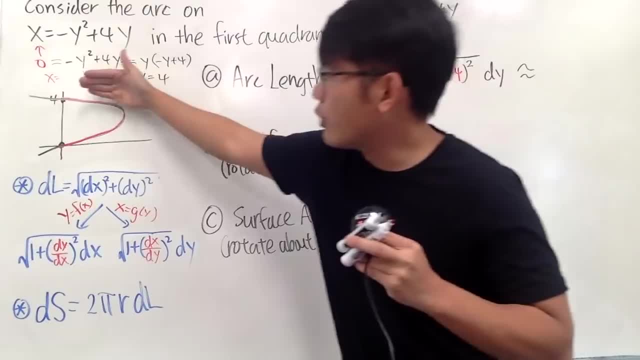 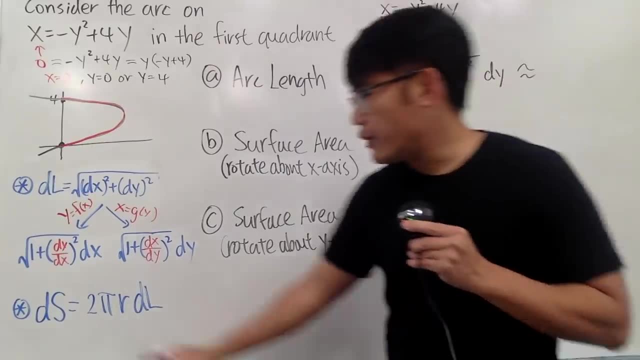 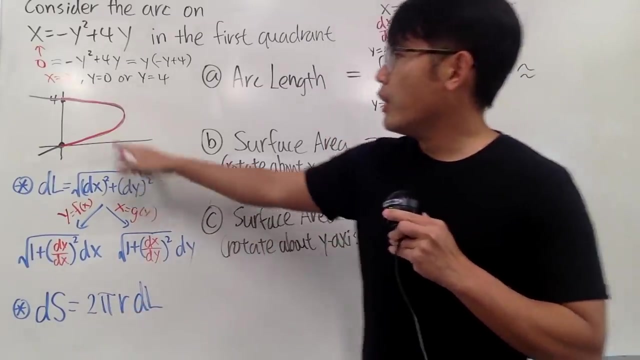 This kind of shape And then the surface area. you have the outer part and then you also have the inner part, right? But anyway, for the surface area, first we have to look at the ds. Formalize 2 pi r times dl r is the radius. Well, if you have a point right here, for example, 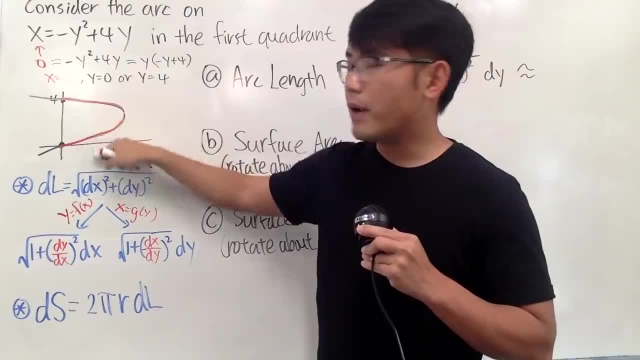 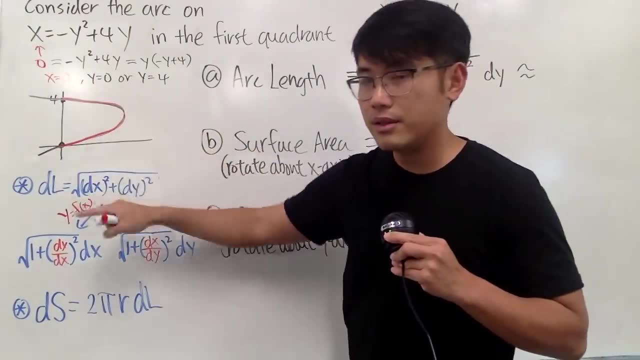 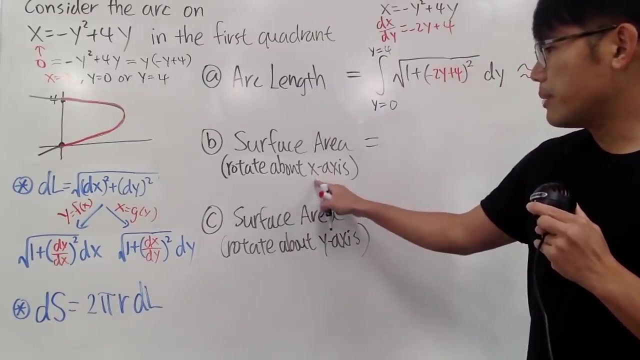 the radius is just going to be the y value because it's vertical. This right here is the y value because you are rotating about the x-axis. So it goes like this: Take this and then rotate, you get the whole thing. So when you rotate about the x-axis, 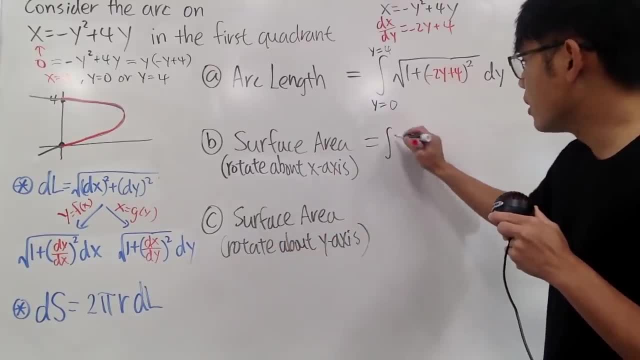 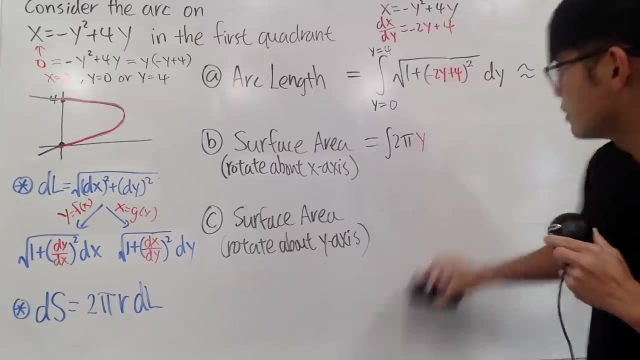 the radius is y, and we just put that down: Integral 2 pi y, and let me also write down the dl for you guys, but in blue though. Let's see if I can hold three markers in one hand like that. 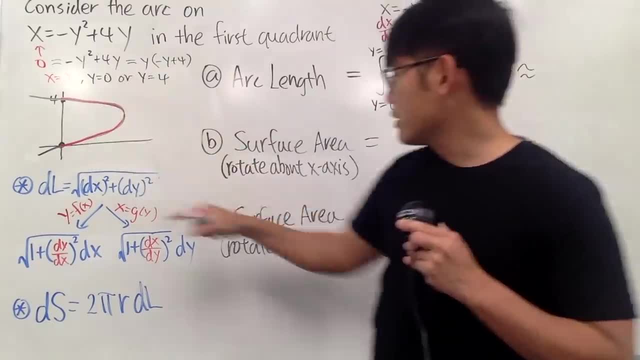 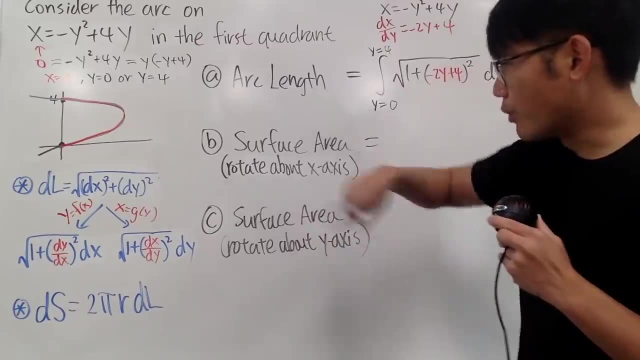 because it's vertical. This right here is the y-value, because you are rotating about the x-axis. so it goes like this: right, Take this and then rotate, you get the whole thing. So for when you rotate about the x-axis, 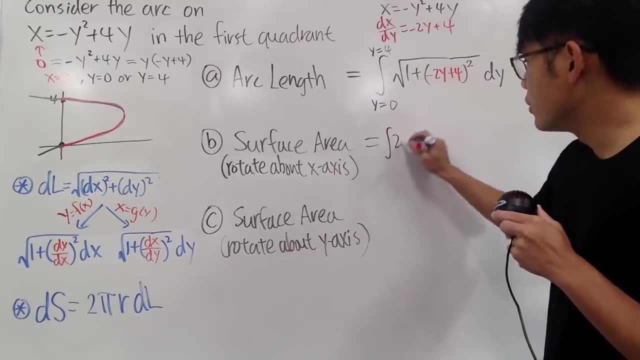 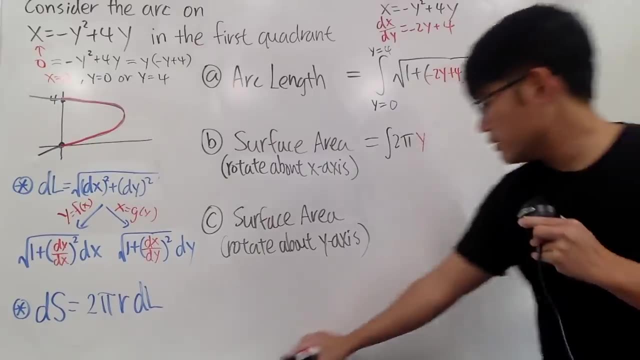 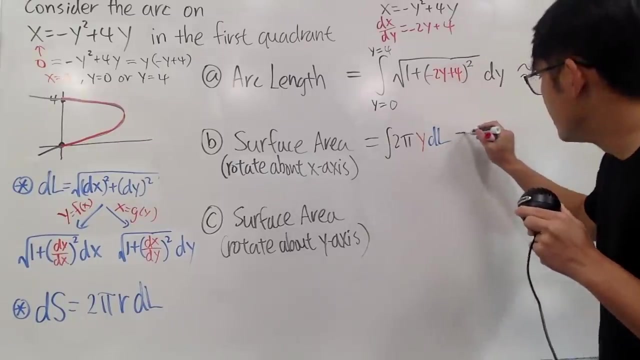 the radius is y and we just put that down: integral 2 pi y. and let me also write down a dl for you guys. Buy Bluedol, Let's see if I can hold string markers in one hand Like that. Now here's the deal. 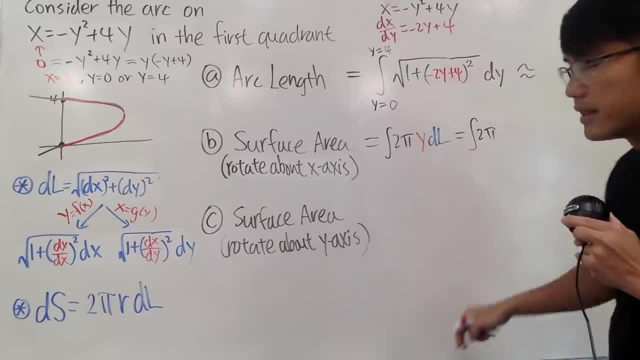 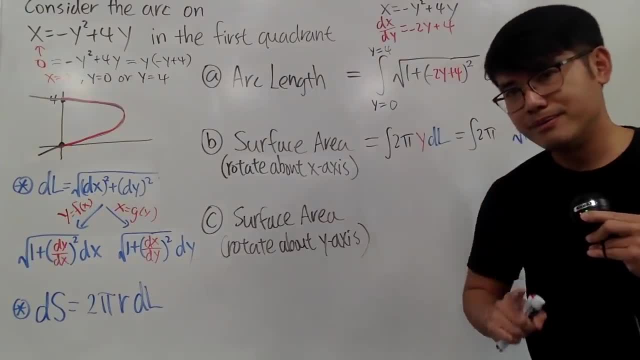 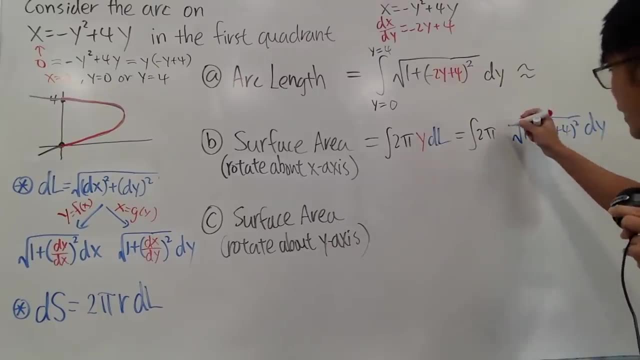 Right, It's the same thing. then we just put that down as how it is now, because we are in the y world, this y, it's totally okay to be right here. so you just go ahead and put down that y as how it is and you're going to pay attention to the y values, which is going from zero to four. 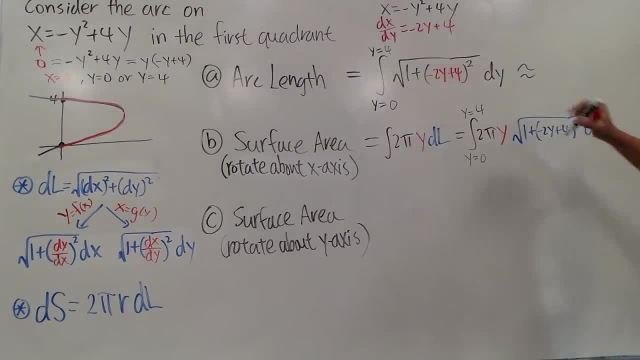 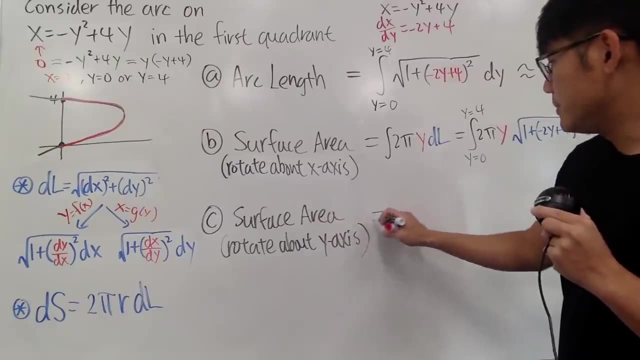 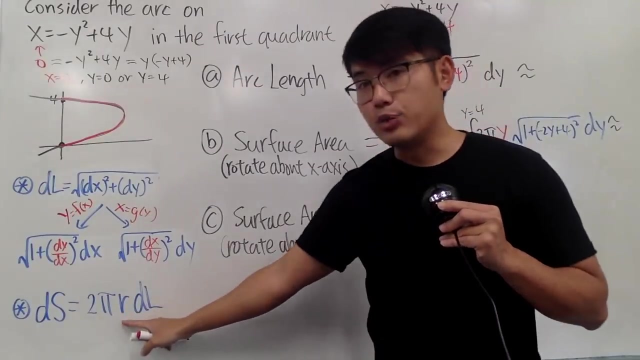 with that we are done. this right here will get you the surface area. when you take the arc rotate about the x-axis. okay, part c: when we take this arc rotate about the y-axis. so it goes like this way: in this case the radius will be the horizontal distance, just put like a point right here, if you. 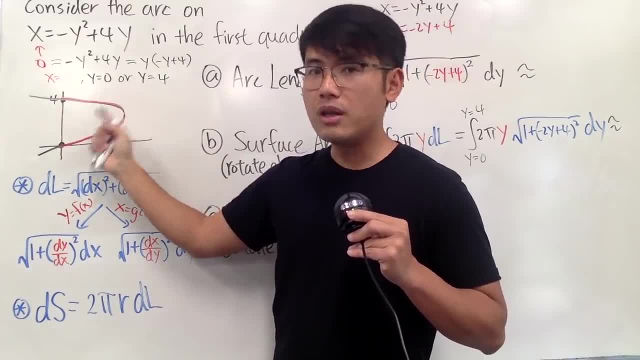 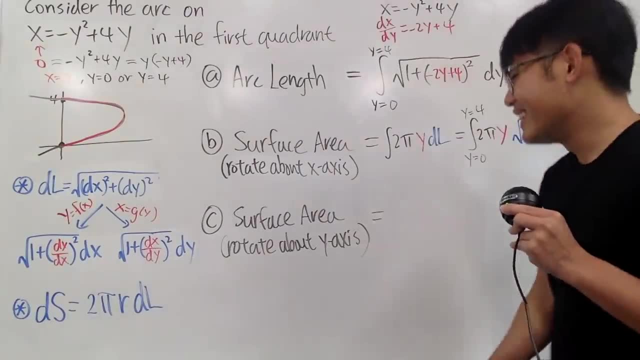 would like go from the y-axis to here. this is the horizontal distance, that's the x value, and when you rotate you know that will be the radius. so let's do the same thing. integral two pi by this is the radius. so let's do the same thing. integral two pi by this is the radius. so let's do the same. 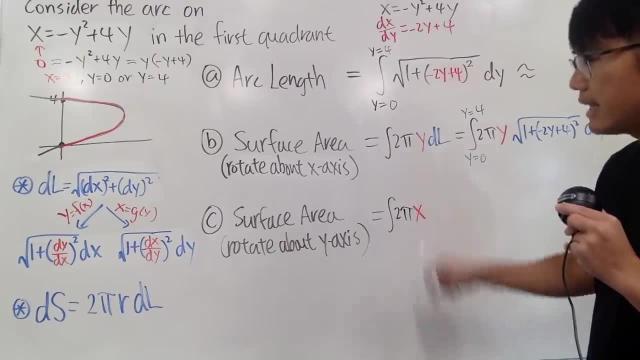 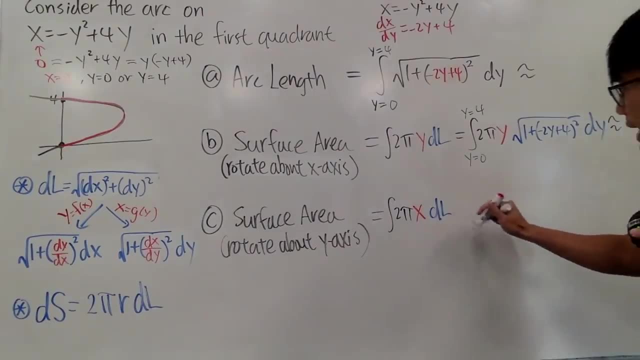 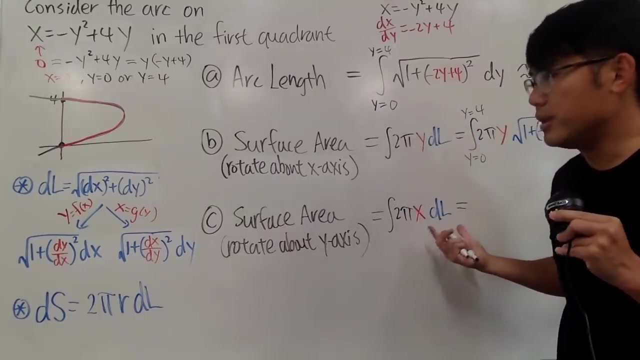 time is x right, two pi x, and we have to have the d l again, and we'll see that so far we cannot finish the integral yet we cannot put down the limits of integrations, because dl doesn't really make that much sense. i don't know which world i'm in yet. 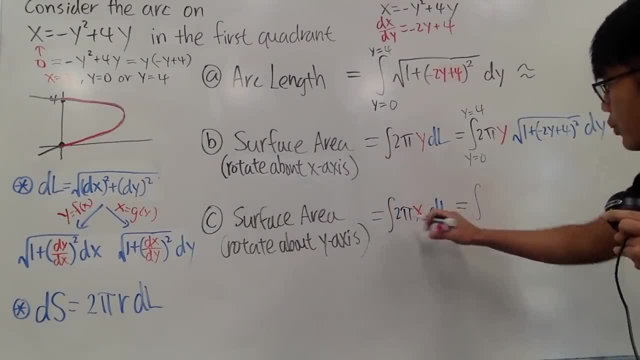 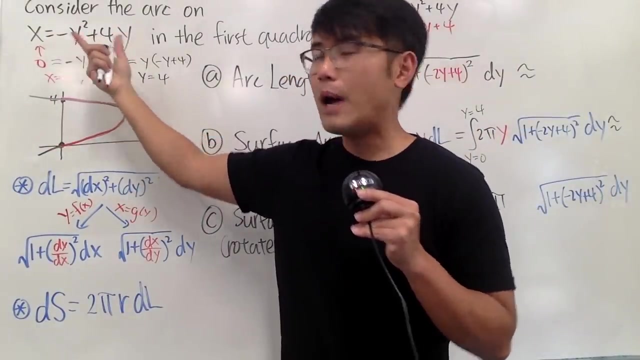 right, all right. put down, the integral: 2 pi is 2 pi. of course, d, l again it's this. so we'll just write that down right here. now. here's the deal: x it's not invited in the y world, but it's okay because we know x and y are best friends, because x is equal to this. so i will just 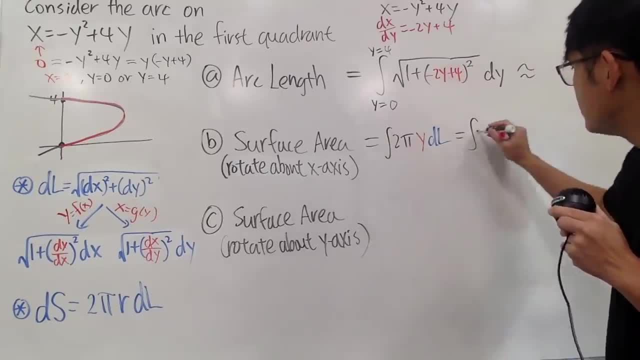 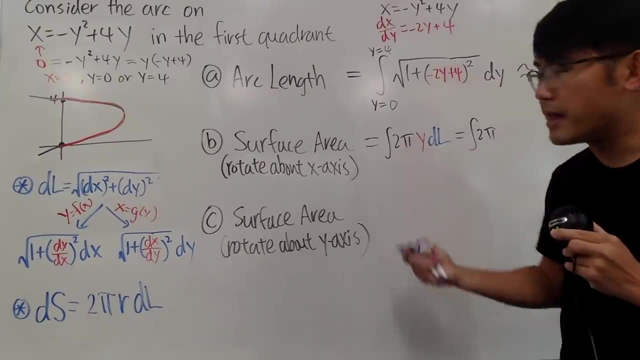 Now here's the deal: Integral is still integral, 2 pi is still 2 pi. Let's put the dl first. dl is from part A, of course. right, It's the same thing. Then we just put that down. 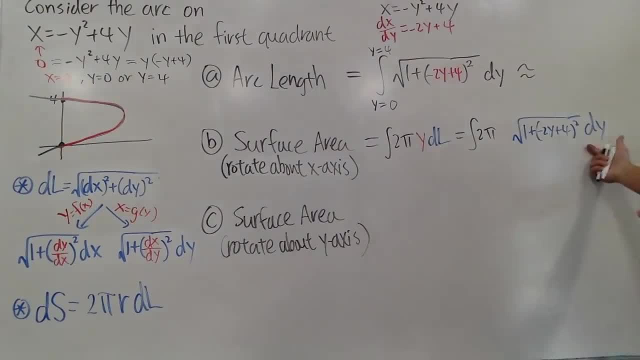 as how it is Now. because we are in the y world, this y is totally okay to be right here. So you just go ahead and put down that y as how it is And you are going to pay attention to the y. 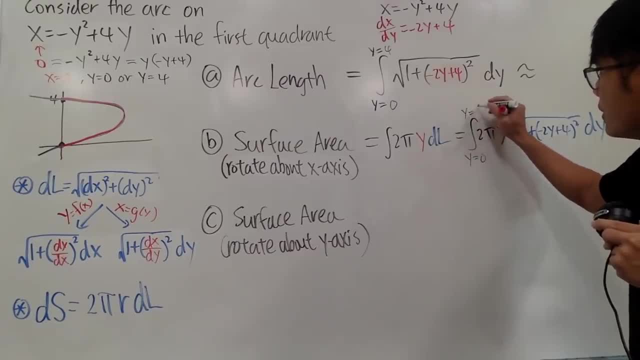 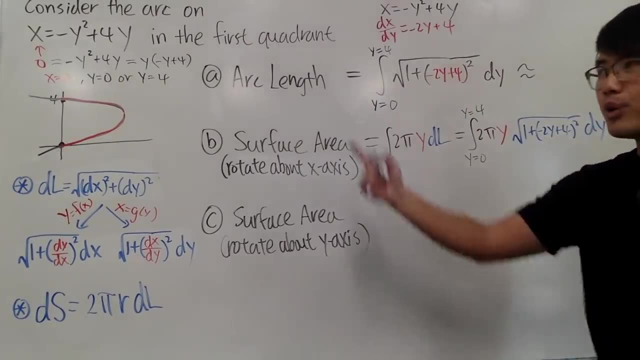 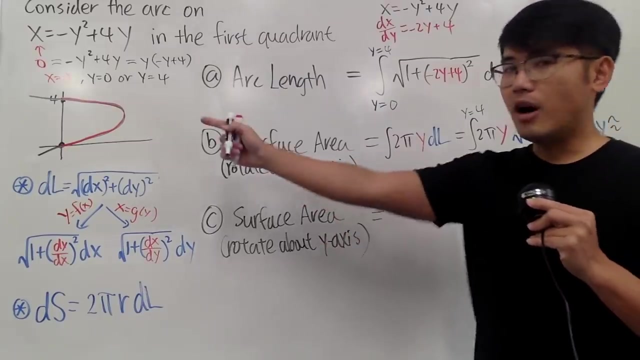 values, which is going from 0 to 4.. With that we are done. This right here will get you the surface area. when you take the arc rotate about the x-axis- Okay, part C. When we take this arc rotate about the y-axis. 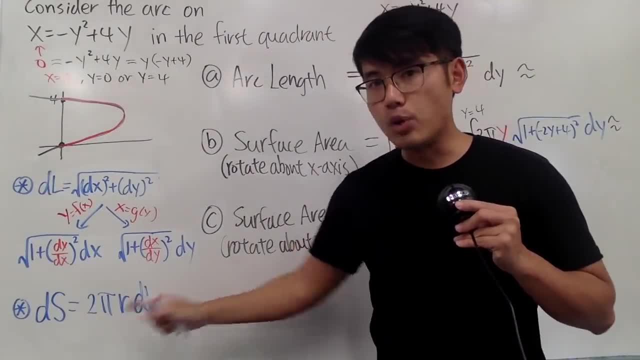 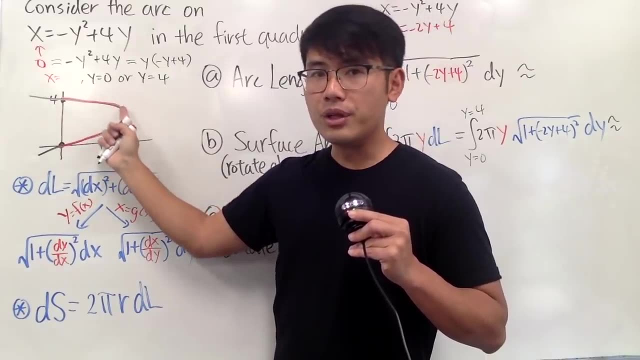 So it goes like this way. In this case, the radius will be the horizontal distance. Just put like a point right here, if you would like Go from the y-axis to here, This is the horizontal distance, That's the x value. 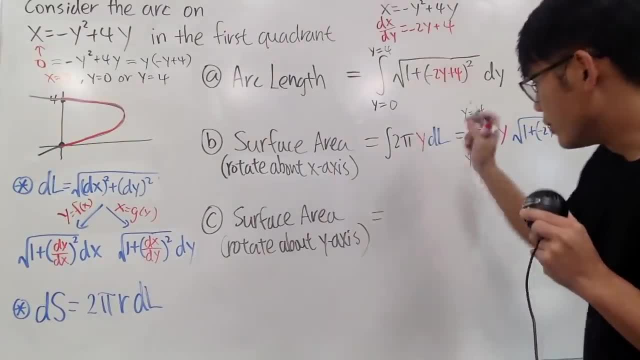 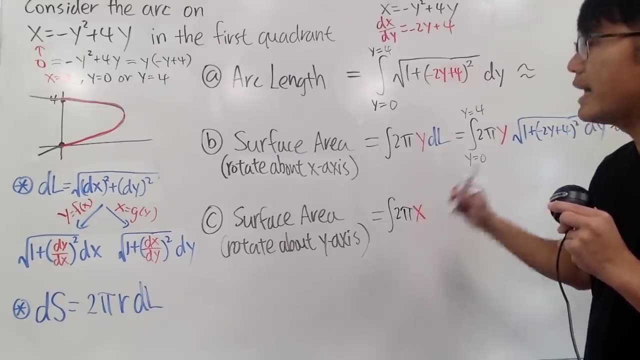 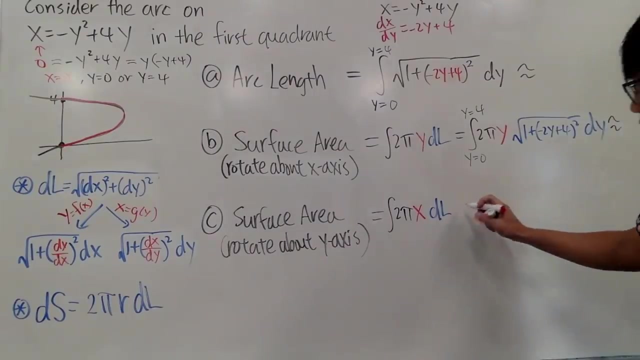 And when you rotate that will be the radius. So let's do the same thing: Integral 2 pi. but this time it's x 2 pi x And we have to have the dl again And we'll see that so far we cannot finish the integral yet. 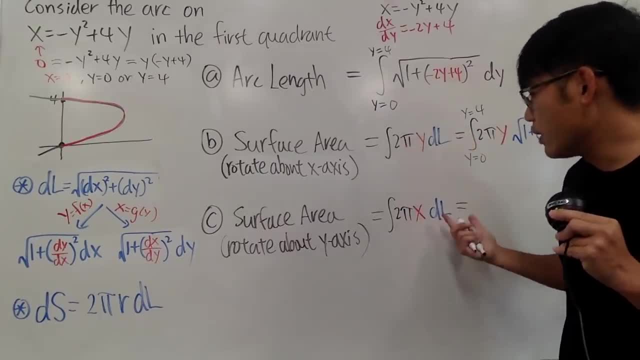 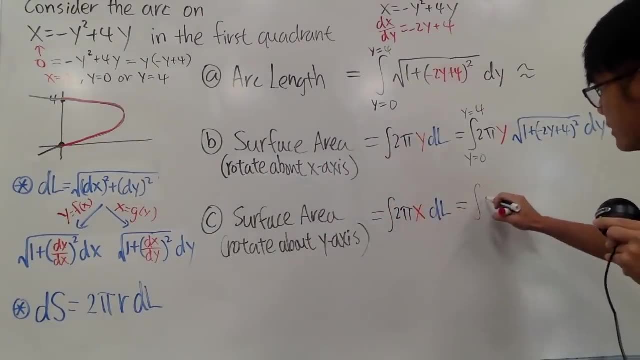 We cannot put down the limits of integrations, because dl doesn't really make that much sense. I don't know which world I'm in yet right, All right, put down the integral 2 pi is 2 pi, of course. 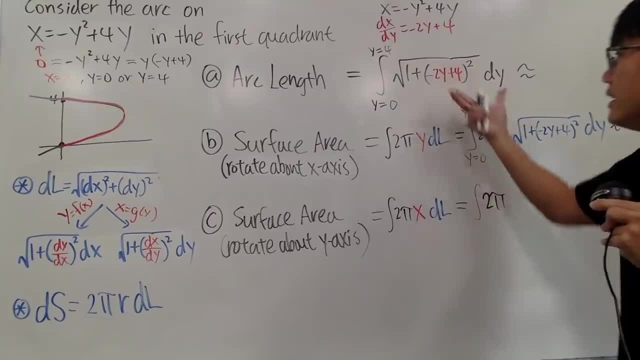 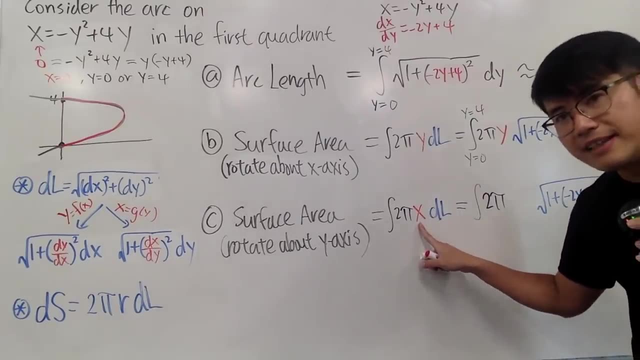 So dl again, it's this, So we'll just write that down right here. Now here's the dl x. it's not invited in the y world, But it's okay because we know x and y are best friends. 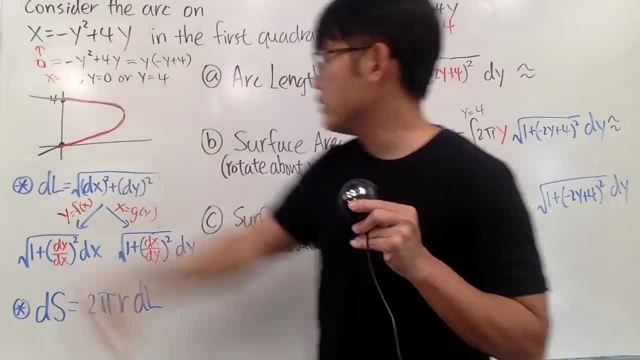 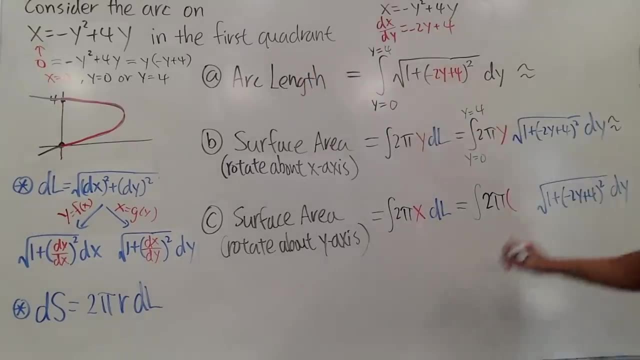 Because x is equal to this. so I will just put this down for the x. We must make that change right, Don't forget about that. So I'll open the parentheses and write down: negative y squared plus 4x. So negative y squared plus 4y. 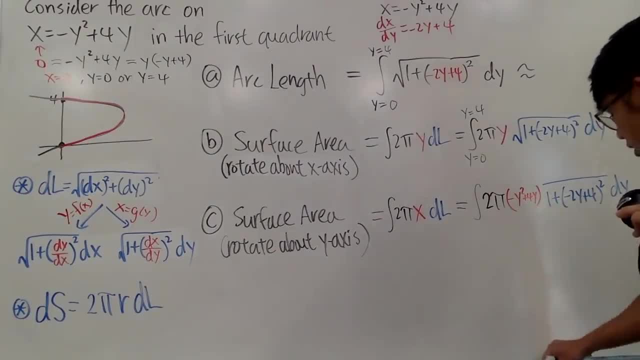 And seriously take some time to use your calculator, Make sure you know how to enter everything carefully and accurately and get your approximation and all that In the end. the final touch is y again goes from 0 to 4.. 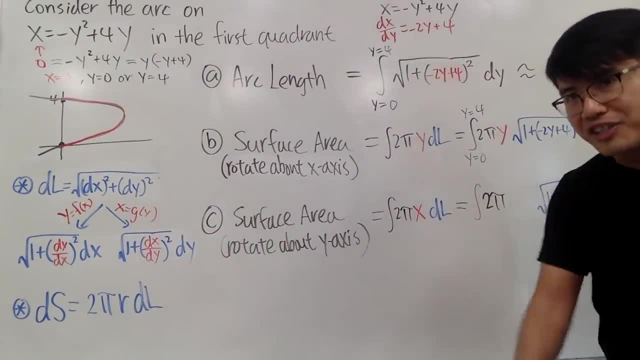 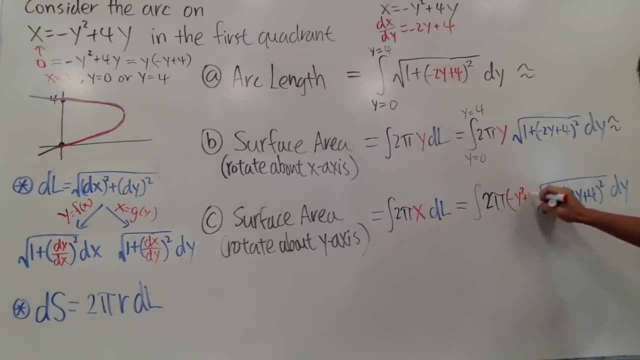 put this down for the x. we must make that change right, don't forget about that. so i'll open the and write down negative y square plus 4y and seriously take some time to use your calculator. Make sure you know how to enter everything carefully and accurately. 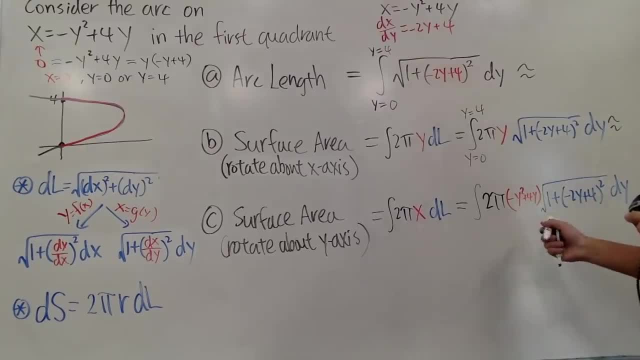 and get your approximation and all that In the end. the final touch is y again goes from 0 to 4. And I'll wait for you guys to tell me the answer. I don't know if you guys can see, but I'm waiting for your approximation. 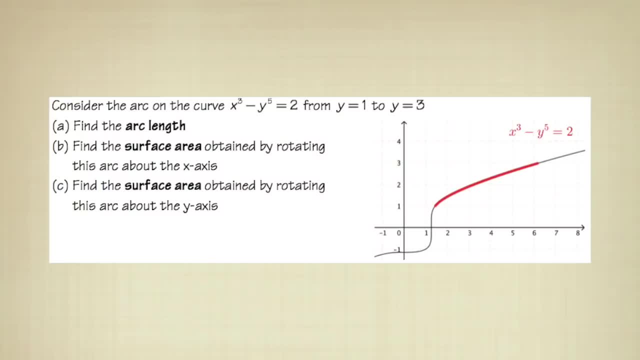 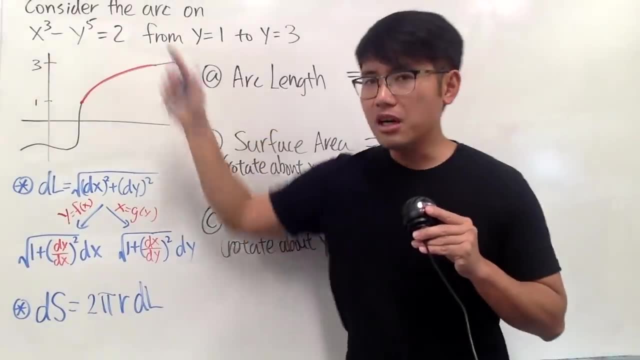 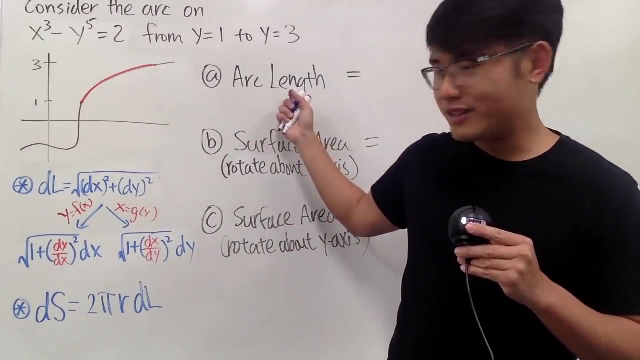 Okay, we are still going to do these three questions, But this time the curve is slightly different, because y is not isolated, x is not isolated, right. So to find the outlinks, of course we have to have one of these situations. 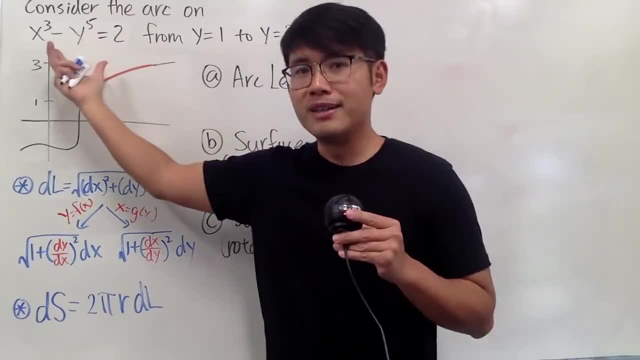 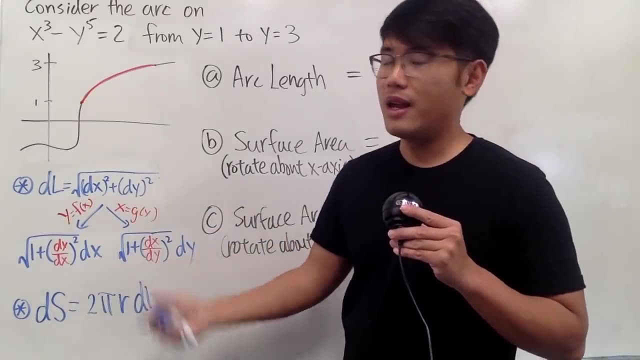 Well, well, it's okay. It's not that bad, because we can do some algebra right here, So we are still good, right. But here's the deal. Which one should we isolate though, The x or the y? Well, we were given that y is going from 1 to 3.. 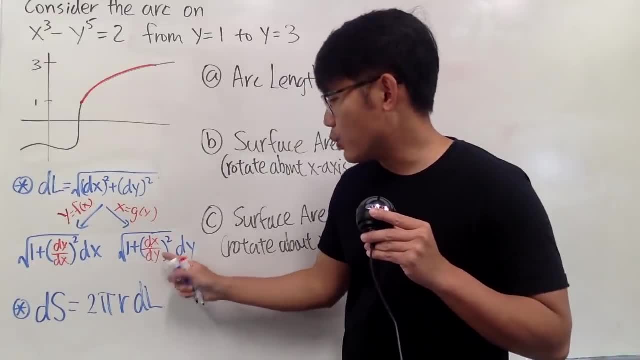 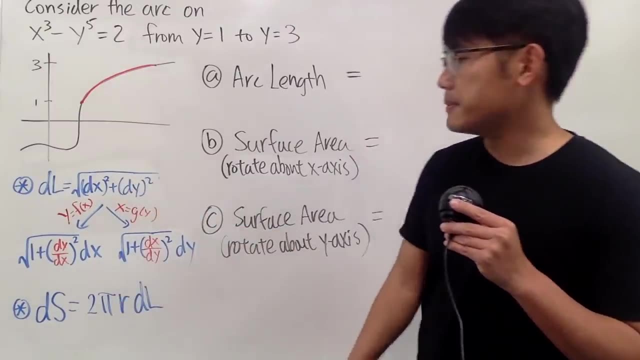 So that means we should be in the y world, right? Because when you have the dy, that means the integral is set up to go from y to the first number to the second number. for the y, That means we should get the x by itself. 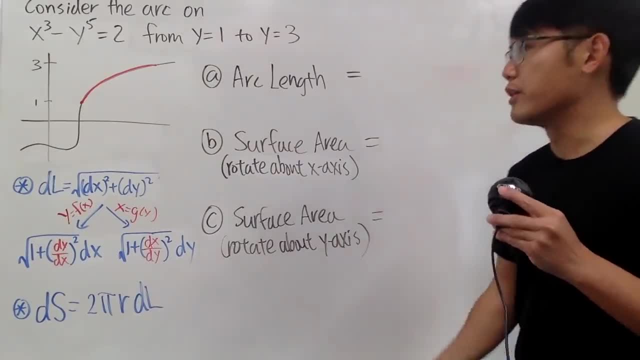 So let's make that happen and then do our derivatives and then do the rest of the questions. So here we go. Of course we can add this on both sides. So we can add this on both sides. So we can add this on both sides. 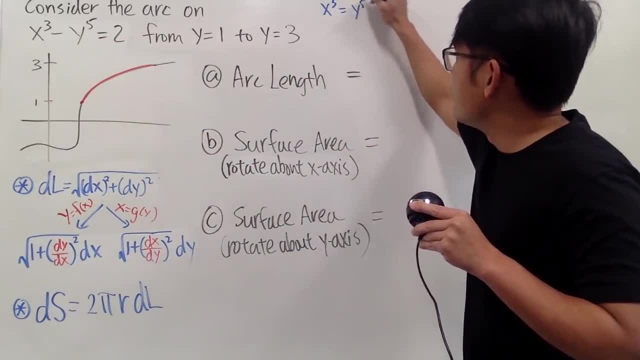 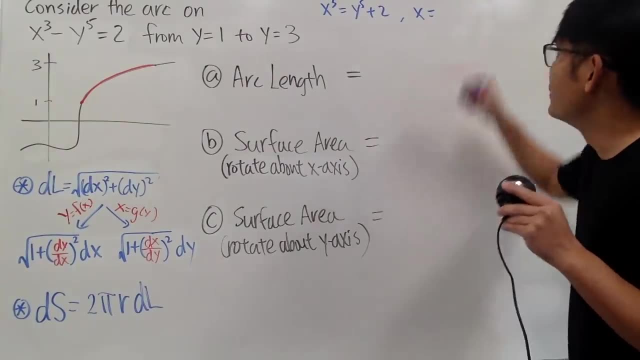 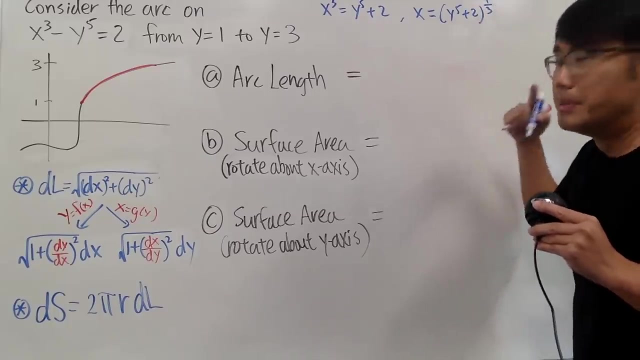 So we can get x cubed equals y to the fifth power plus 2.. And we will just take the cube on both sides. So this means x is by itself now And we get- let's write it as y to the fifth plus 2, raised to the one-third power. 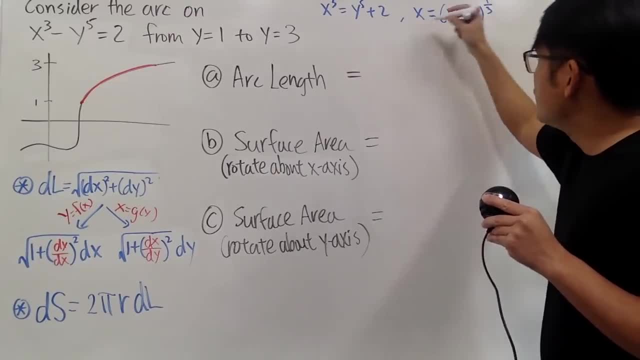 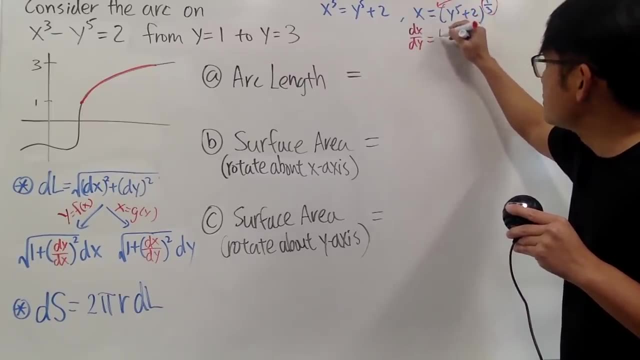 Because we have to do our derivative. when we do our derivative, by looking at this form, we get dx dy being. bring this to the front. so we have one-third. We put states the same, which is y, to the fifth plus 2.. 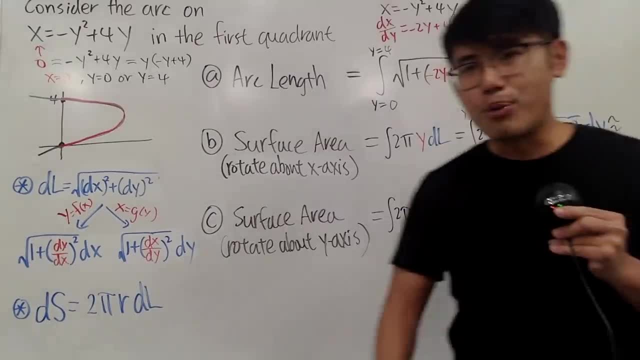 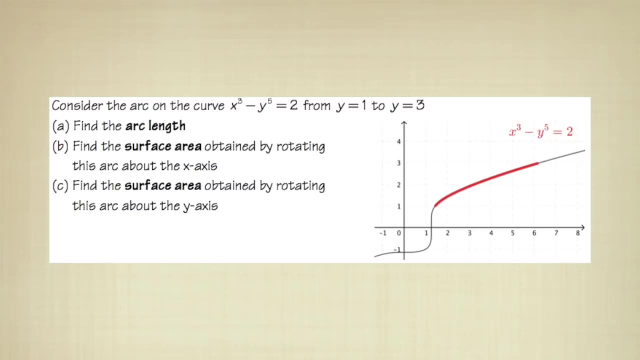 And I'll wait for you guys to tell me the answer. I don't know if you guys can see, but I'm waiting for your approximation. Okay, we are still going to do these three equations, but this time the curve is slightly. 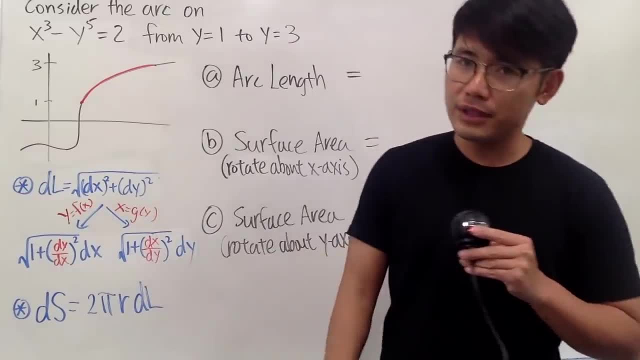 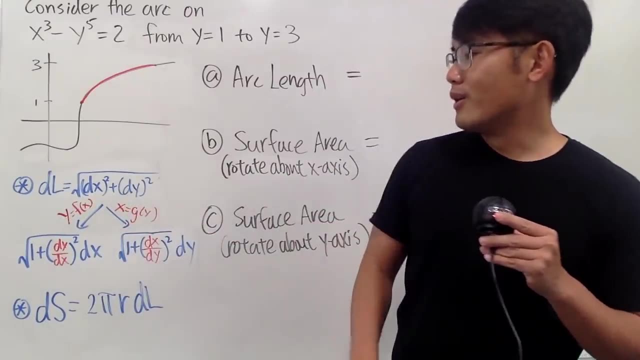 different because y is not isolated, x is not isolated, right. So to find the arc length, of course we have to have one of these situations. Well, well, it's okay, it's not that bad, because we can do some algebra right here. so we are. 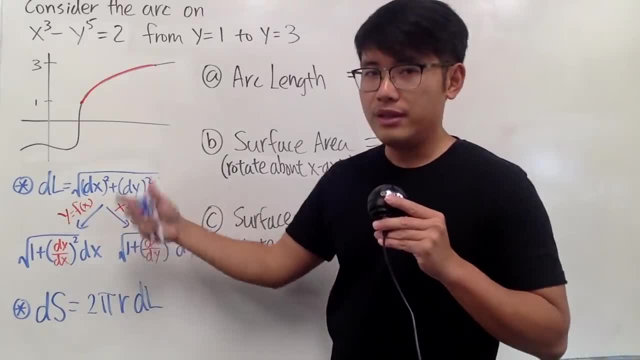 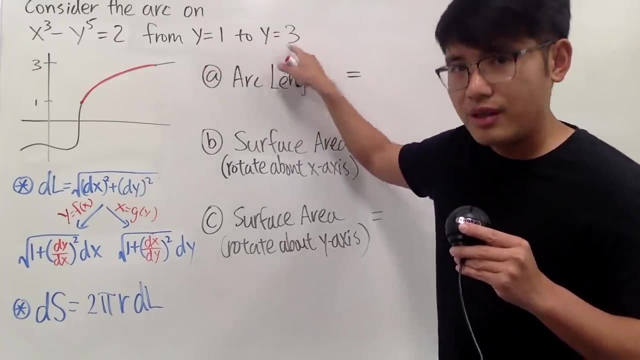 still good, right. But here's the deal. which one should we isolate though, the x or the y? Well, we were given that y is going from one to three, so that means we should be in the y world, right. 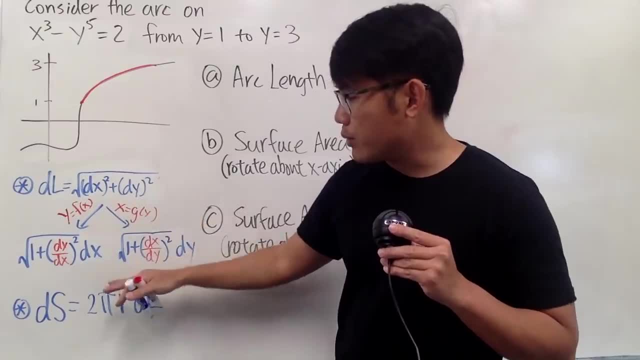 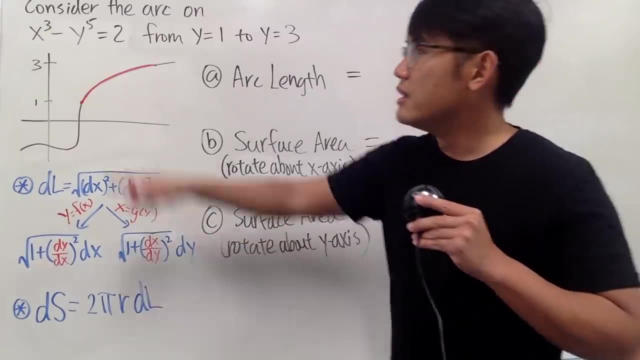 Because when you have the dy, that means the integral is set up to go from y to the first number to the second number. for the y That means we should get the x by itself. So let's make that happen and then do our derivatives and then do the rest of the questions. 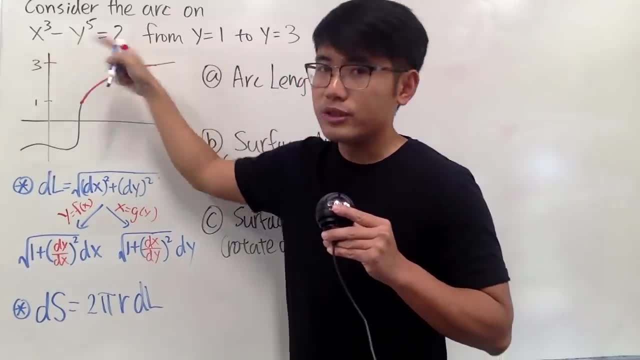 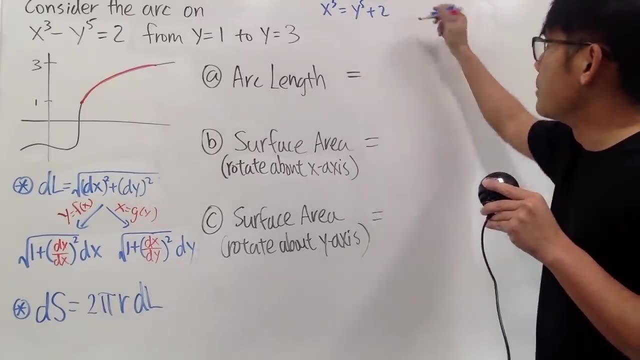 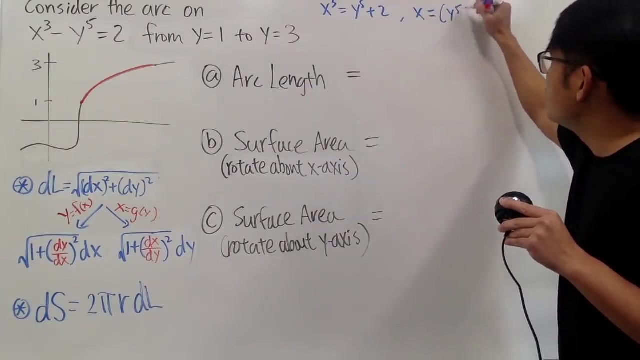 So here we go. Of course we can add this on both sides, so we can get x cubed equal to 0.. Of course, y to the fifth power plus two, and we will just take the cube on both sides. so this means x is by itself now and we get- let's write it as y to the fifth plus two. 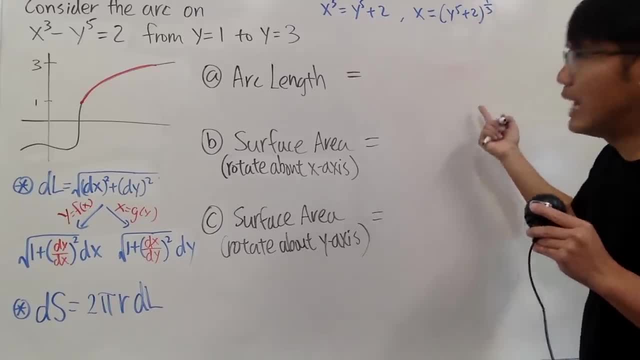 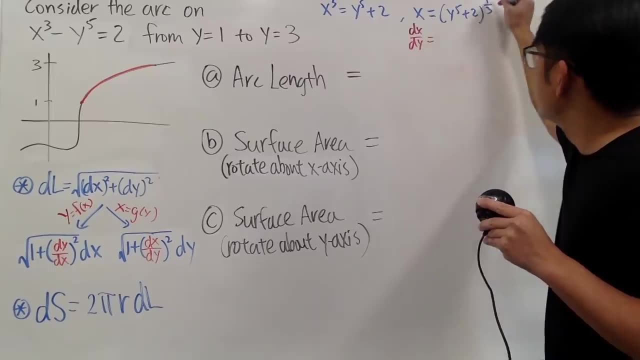 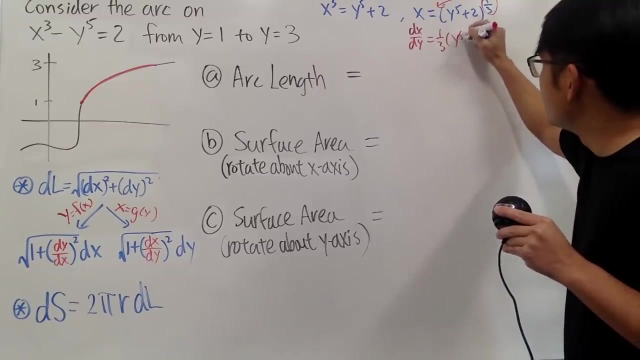 raised to the one-third power Because we have to do our derivative. when we do our derivative, by looking at this form we get dx dy being bring this to the front. so we have one-third and the input stays the same, which is y to the fifth. 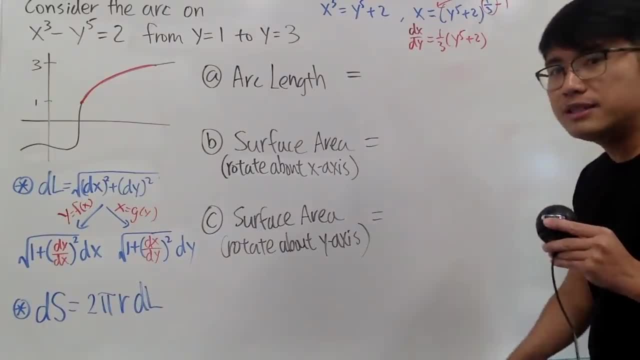 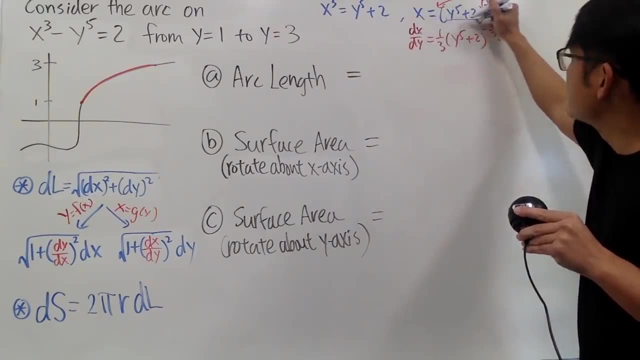 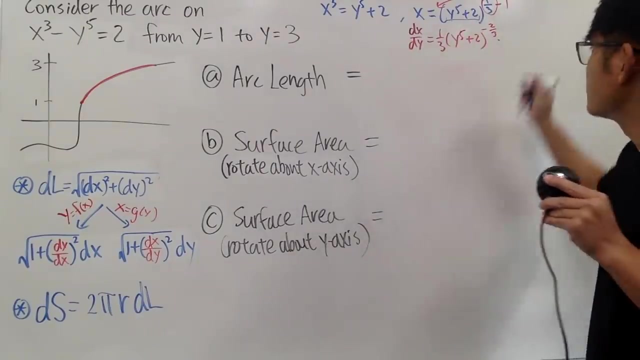 So we get y to the fifth plus two, but don't forget to minus one to the exponent. One-third minus one is negative two-thirds and we multiply by the derivative of the inside because of the Chandu. okay, And the derivative of the inside is five y to the fourth power. so just multiply by it. 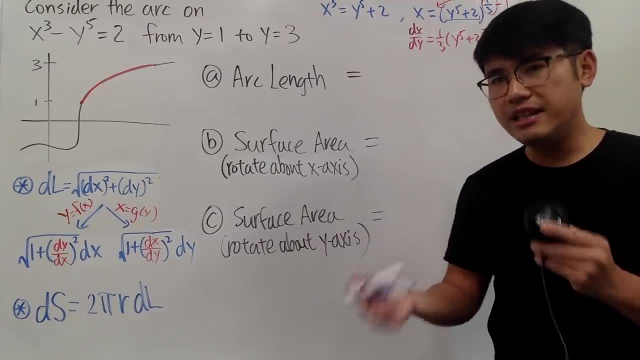 right here And right here there's nothing too much we can simplify, and in the end we'll just be using our calculator anyway. but I do want to put the five on top of this right here, so let me make that happen. 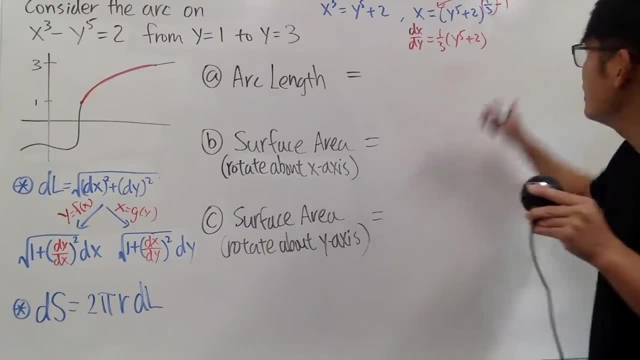 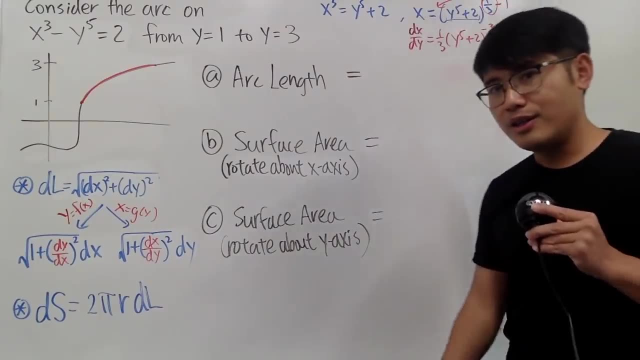 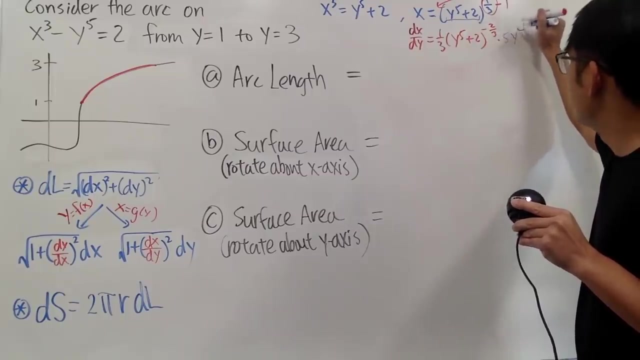 But don't forget to minus 1 to the exponent One-third minus 1 is negative two-third And we multiply by the derivative of the inside because of the chandu. okay, And the derivative inside is 5y to the fourth power. so just multiply by it, right here. 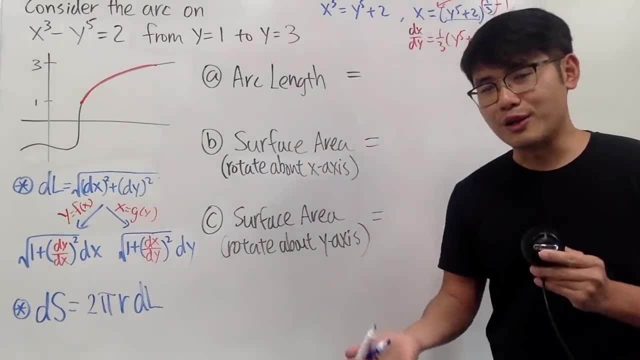 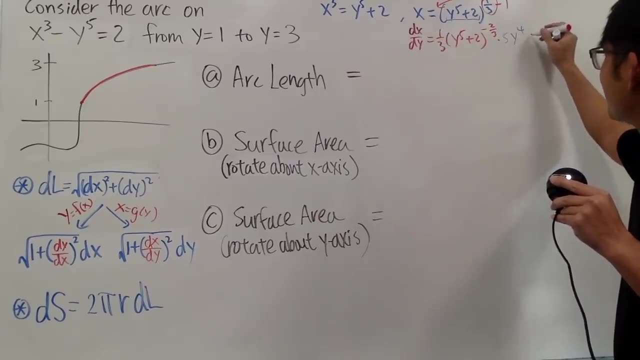 And right here there's nothing too much we can simplify, And in the end we will just be using our calculator anyway, but I do want to put the top of this right here, so let me make that happen. so this right here is just 5 over 3, and let's 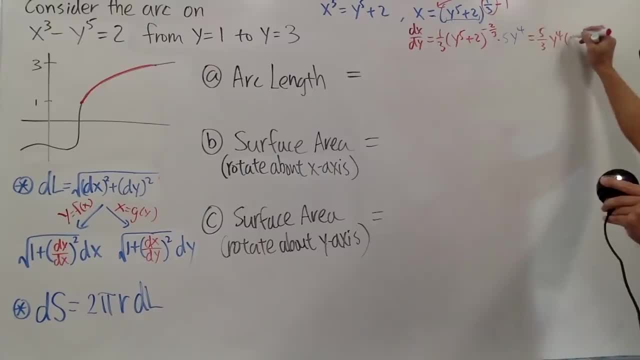 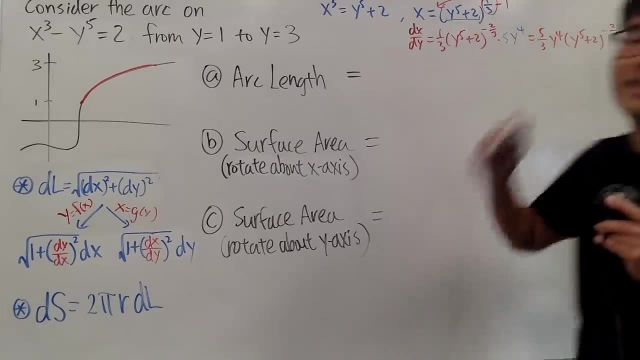 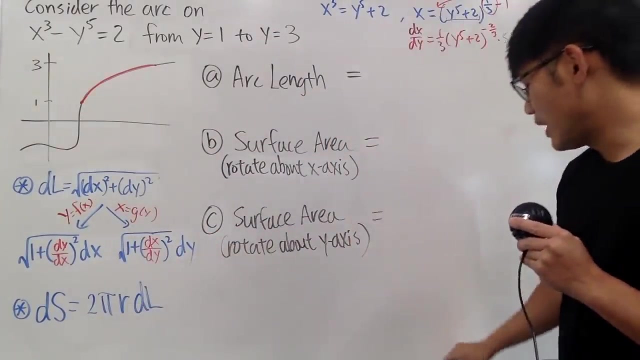 write down the y to the fourth power first and all this, and let me just write it down like this. it's easier to put it down like this on the calculator. so this right here will be our derivative. now our length in action will be using this version. so here we go. we have to have the 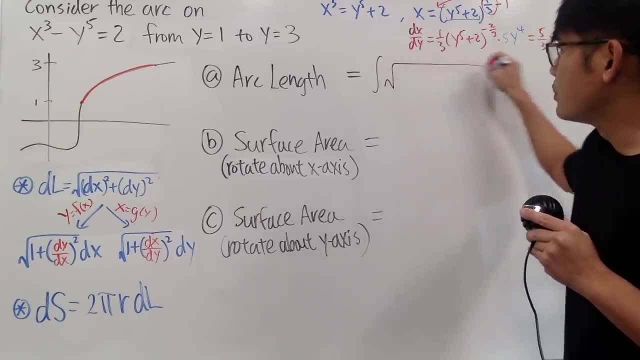 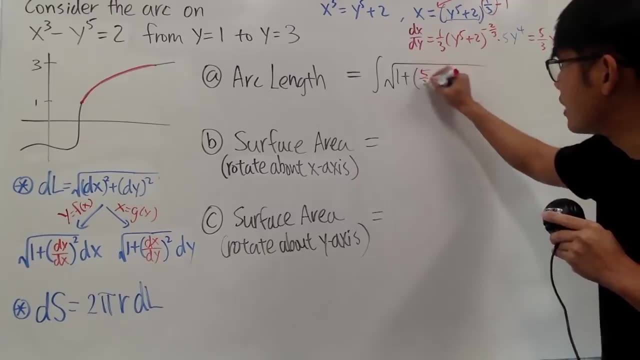 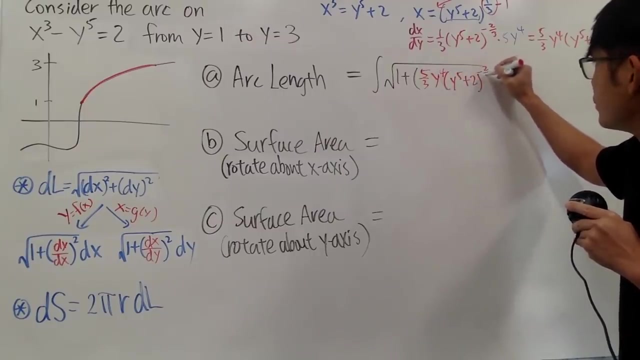 integral, of course. so integral, squared root. one is the one- and we add the parentheses, all that inside here- which is 5, 3rd, y to the fourth power times, y to the fifth power, plus two raised to the negative, 2, 3rd power. and this right here is the derivative, and we are just going to. 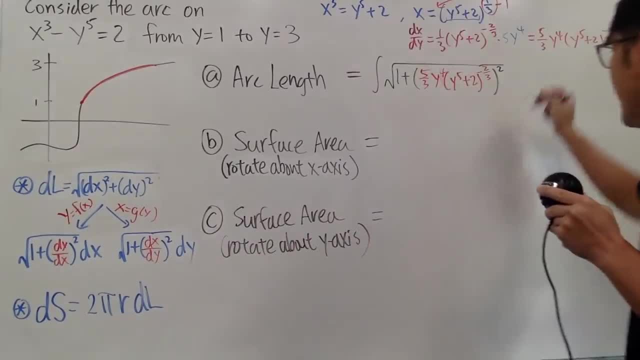 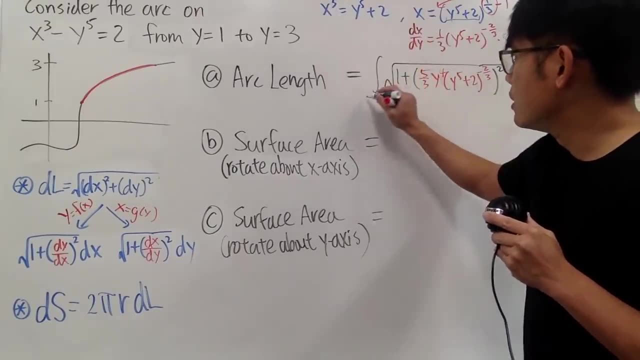 take this and raise to a second power, because the formula says so and we have the dy here and dy right. so we have, we have in the y-world, we have to go from 1 to 3.. And again, if you really want to, you can. 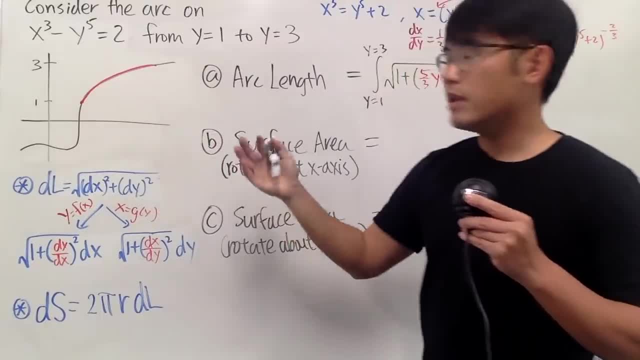 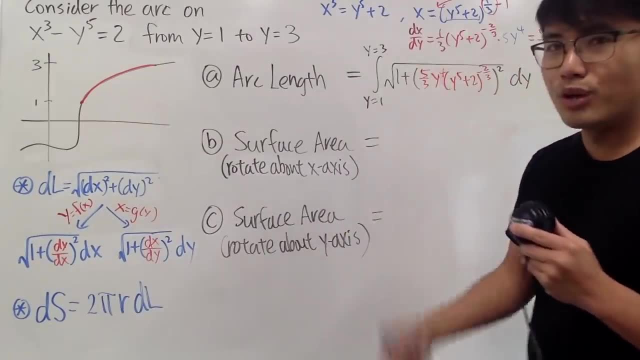 actually put in the y into the original equations and you can get the x values and you can actually use this one if you would like, and you can get the y by itself. that stuff. It's just easier this way, slightly more convenient. Alright, next we have to have the surface. 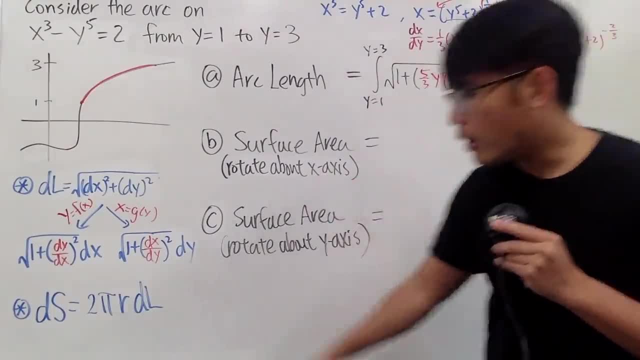 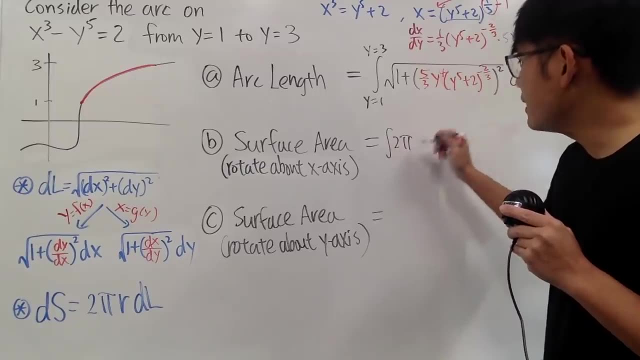 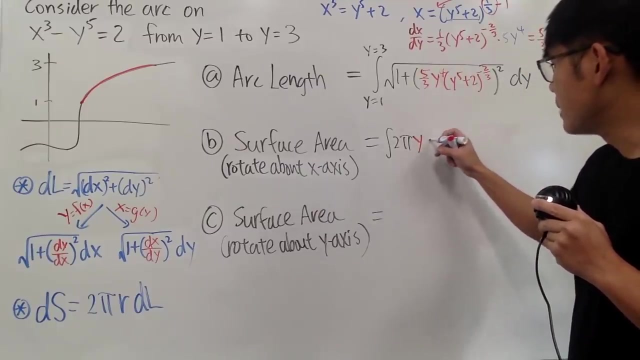 area. Well, rotate about the x-axis. we know the radius will be the y value, So we will have the integral of 2 pi and then the y, and we also have to have the dl. The dl is just all that, so it's not that bad. Now check this out. I'm about to put in all this. 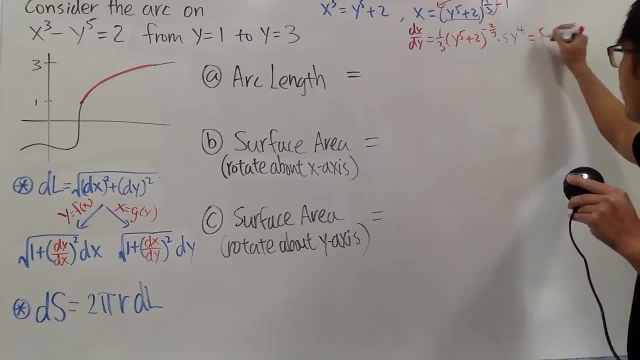 So this right here is just five over three, and let's write down the y to the fourth power first and all this. And let me just write it down like this. it's easier to put it down like this on the calculator. So this right here will be our derivative. 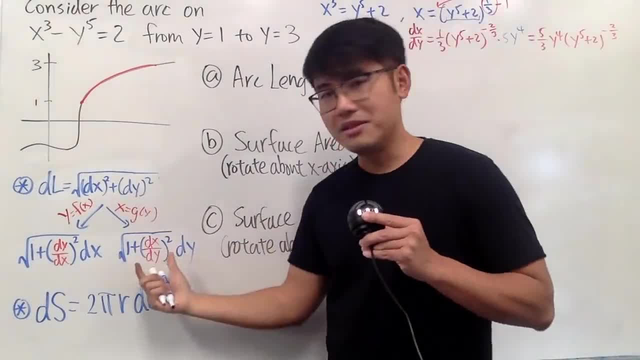 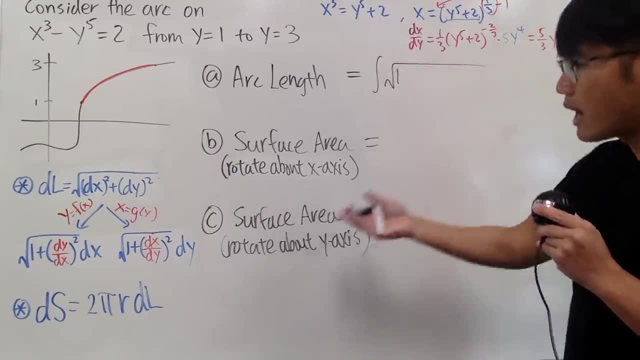 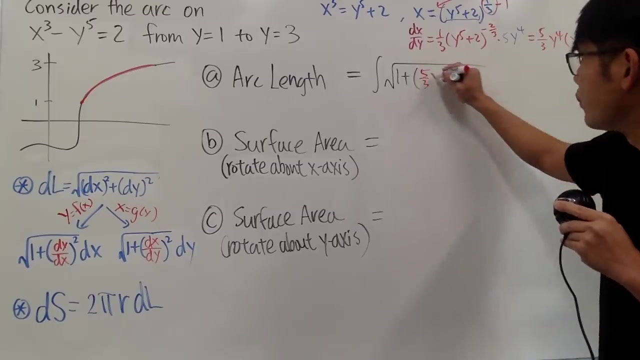 Now our length in action. we'll be using this version, So here we go. We have to have the integral, of course. So integral square root one is the one, And we add the present, Add the parentheses, all that inside here, which is five third y to the fourth power. 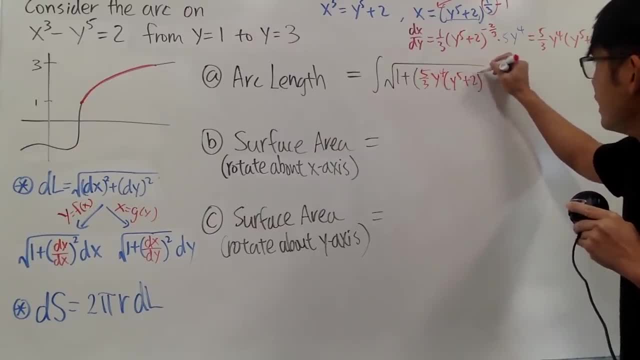 times y to the fifth power plus two raised to the negative two third power. And this right here is the derivative And we are just going to take this and raise to a second power because the formula says so And we have the dy here and dy right. 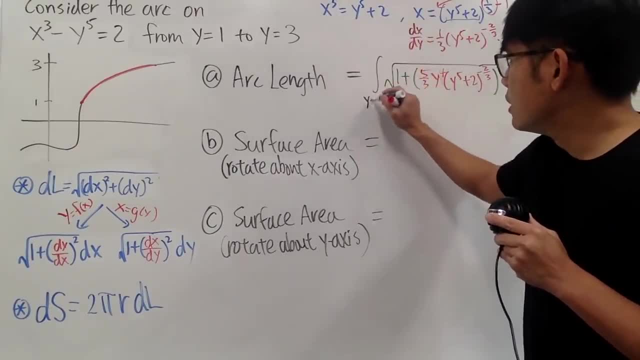 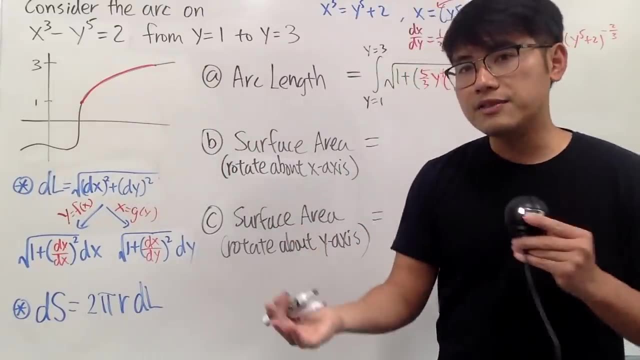 So we are in the y world. We have to go from one to three. And again, if you really want to, You can actually put in the y into the original equations and you can get x values and you can actually use this one if you would like, and then you can get the y by itself. that, 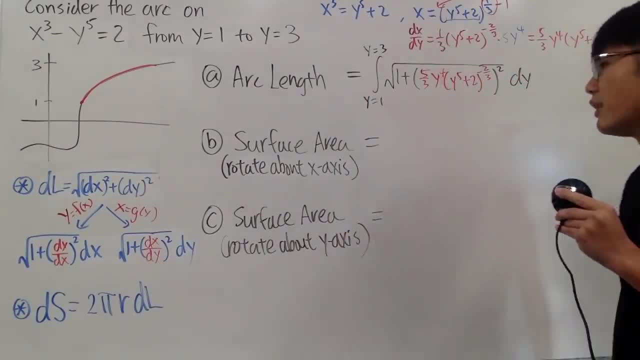 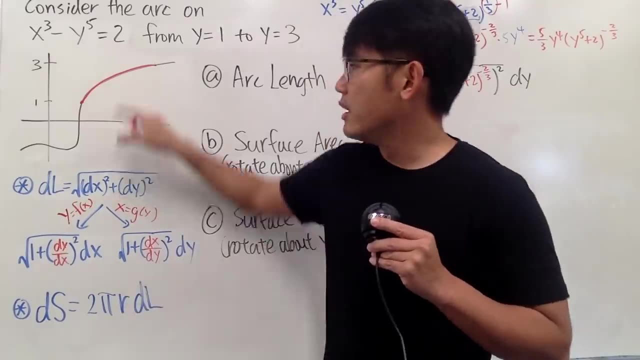 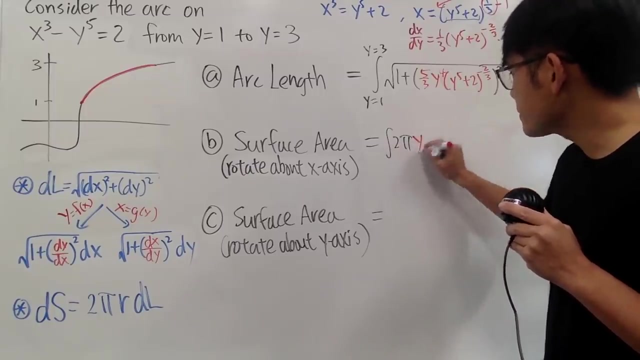 stuff. It's just easier this way. It's slightly more convenient, All right. Next we have to have the surface area Well rotate about the x axis. we know the radius will be the y value, So we will have the integral of two pi and then the y. 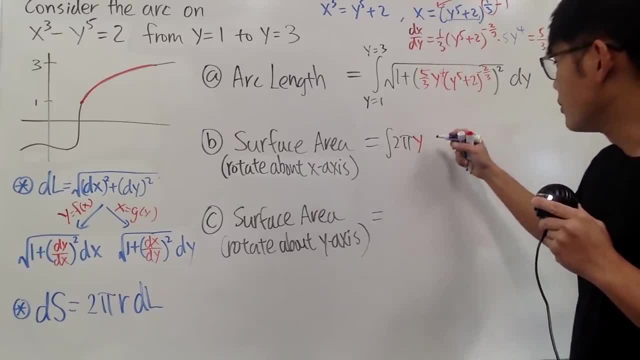 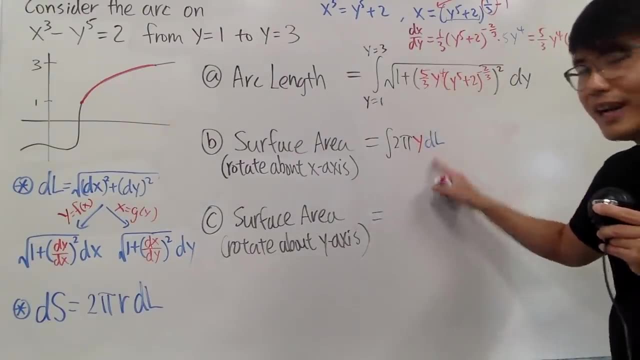 And we also have to have the dl. The dl is just all that. So we have the y, So it's not that bad. Now check this out. I am about to put in all this for the dl, right, So the y is actually good. 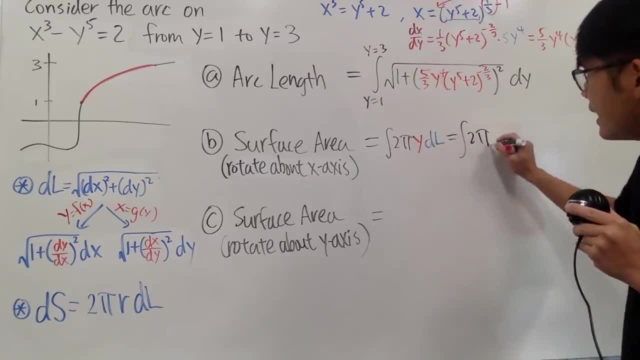 Anyway, we'll see. this is the integral two pi And let me just write down the dl. all this right here in blue, And we have to have the y, which is just the y, because y is invited in the y world. 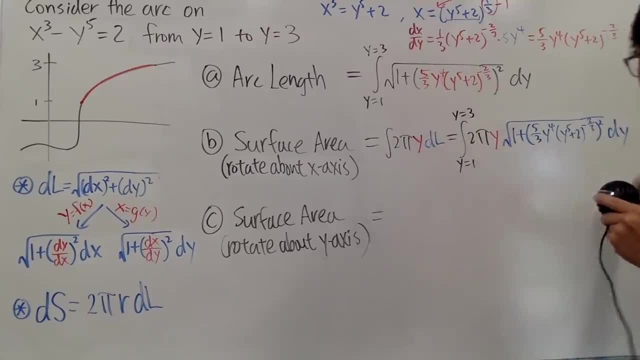 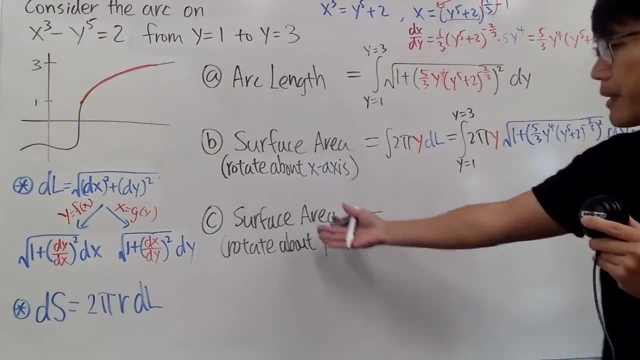 Cool, And y goes from one to three. So this is nice Done And, just like the other ones, you are going to tell me what the approximation is. Now. the surface area, when you take the arc, rotate about the y axis. in that case, the